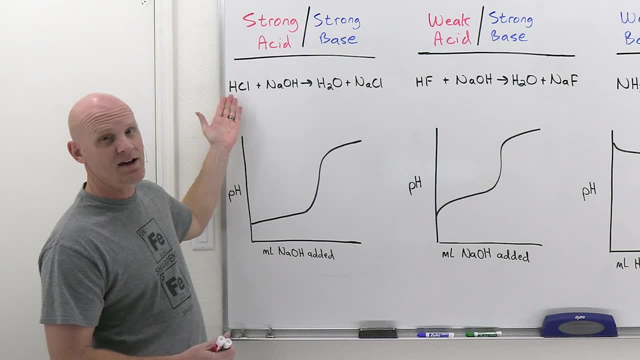 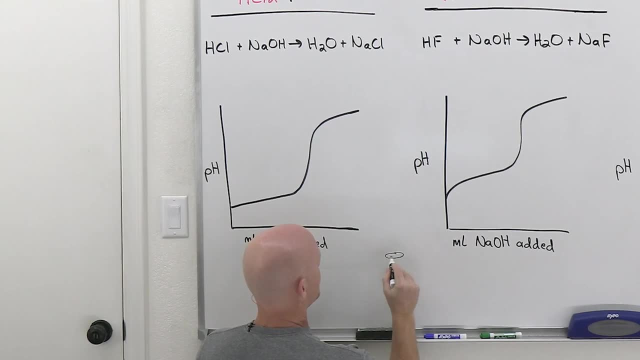 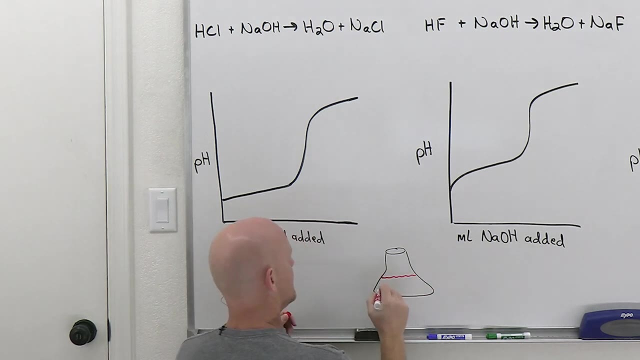 acidic or basic species. In our case, we're going to make that species the HCl. We're going to try to determine the concentration of HCl in here, And so what we would typically do is we'd take a flask So and we put inside that Erlenmeyer flask, our acid solution, and whatever you're. 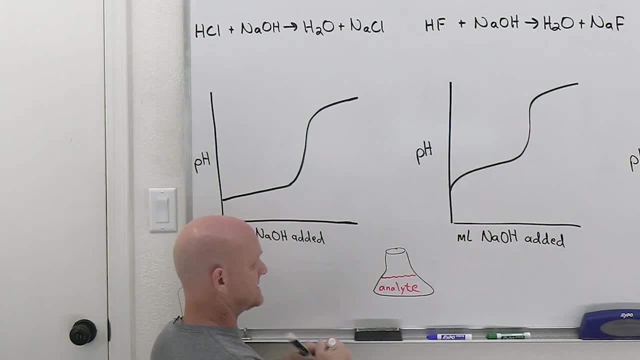 trying to determine the concentration of, we would refer to that as your analyte. So, and then you're going to set up a burette and inside that burette- in this case, if the analyte is an acid, then in your burette is going to be a base And we're going to refer to this guy as your titrant. And 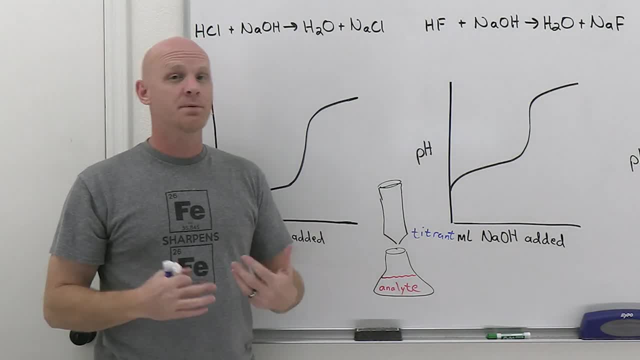 it could be the other way around. If you're, you know, trying to figure out the concentration of the unknown, you know some unknown concentration of a base, well then the base would be the analyte and you'd use an acid as your titrant. So these are two common words. you should definitely 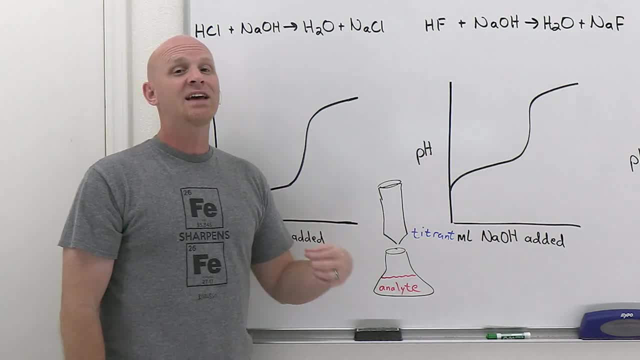 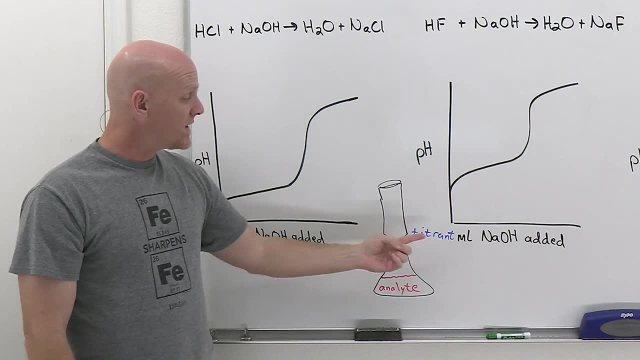 be familiar with. And the key is, the titrant is going to be standardized And by standardizing it, we're going to know its exact concentration. That's going to be important because by knowing its exact concentration, we'll be able to determine the exact concentration of the analyte. 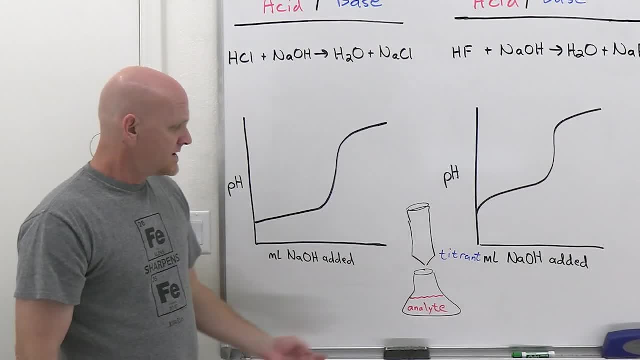 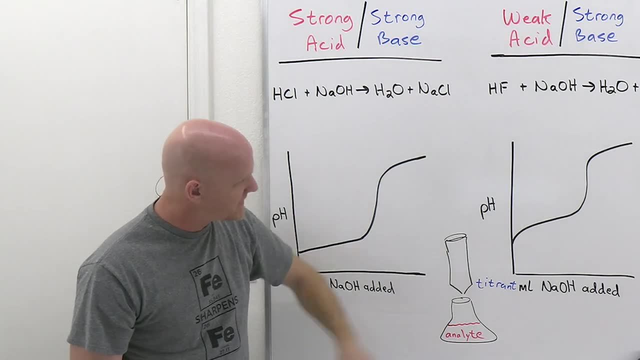 Again, which is usually the whole point of doing a titration. So in this case our analyte is an acid- It's HCl in this example- And so the pH starts out low And as we start shooting NaOH into there, 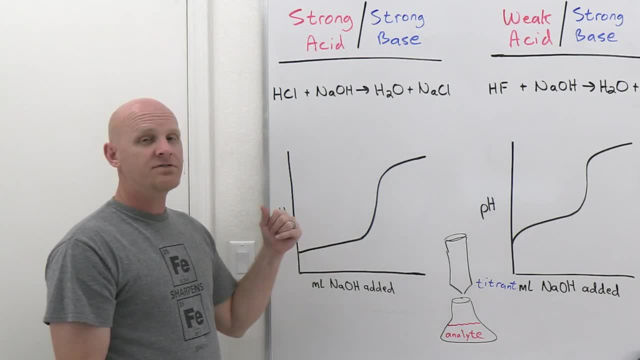 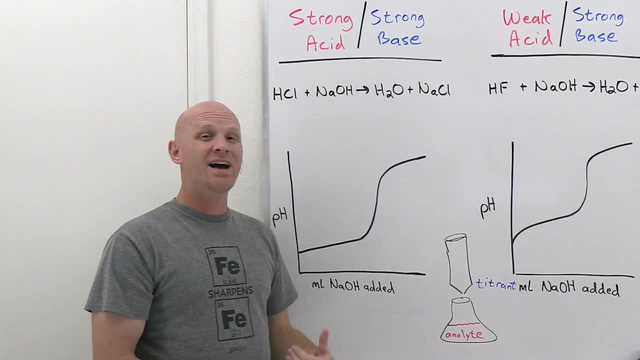 the pH is gradually going to start to increase, But at some point, rather than being a gradual increase, you're going to get this very rapid increase. So from like this point here to this point here might be a difference of only adding a drop or two of NaOH, And the whole point is to 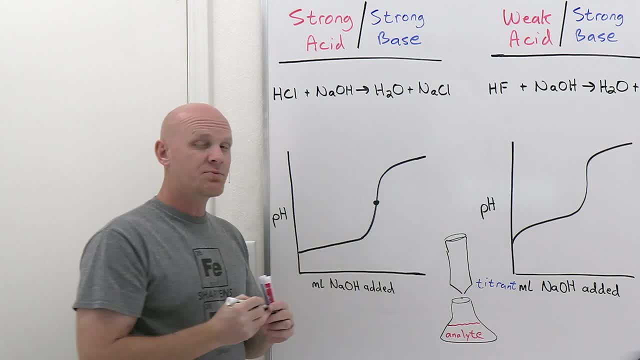 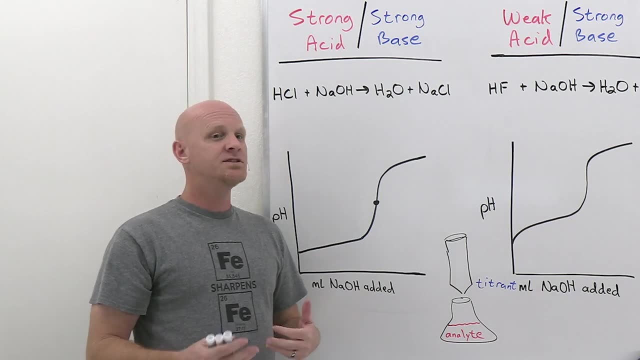 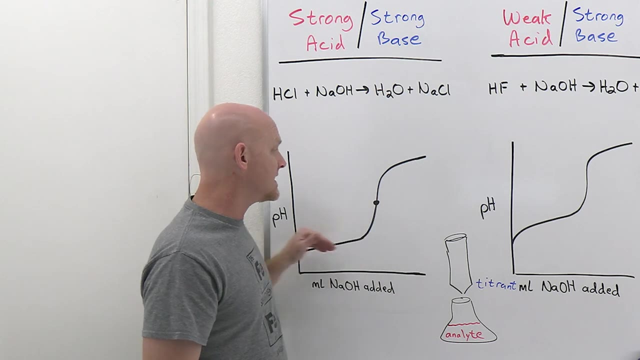 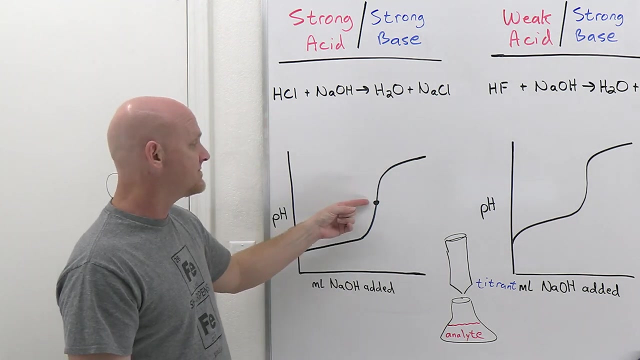 get to this midpoint right here, And I'll call it a midpoint. Really, we should properly call it an inflection point. So at an inflection point is where the slope is either changing from either increasing to decreasing or decreasing to increasing. And so you can see here: all the way up until that point the slope has been gradually increasing, getting more and more steep, But now it's going to change to decreasing, getting less and less steep, And if you're into calculus, that means the sign of the second derivative goes from being positive to negative. Definitely not something you need to know here, But that's an inflection point on this graph. So when you hear somebody refer to this equivalence point as an inflection point, that's what they mean. 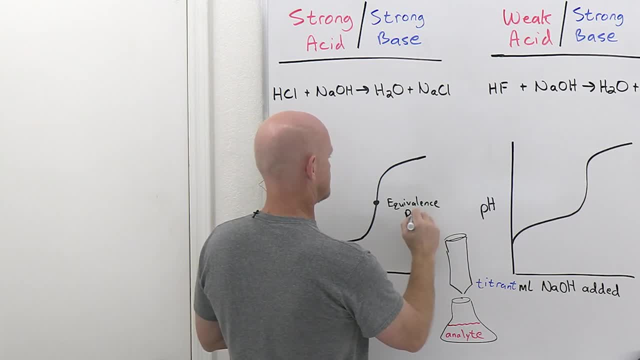 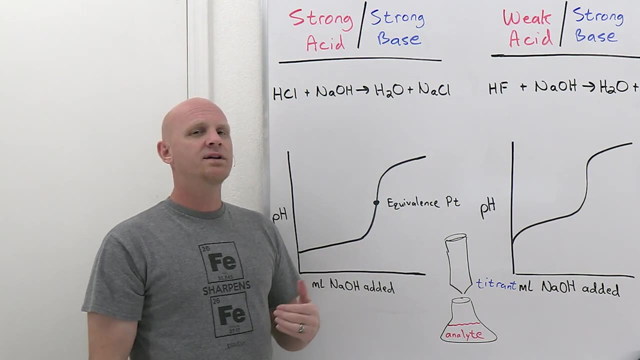 Let's put that out here. So this is the equivalence point. Sometimes we shorten that to EQ point, So and a lot of students forget that it's the equivalence point is not the equilibrium point. So and what we mean by the equivalence point is it is the point at which you've added a chemically equivalent amount of acid or base. 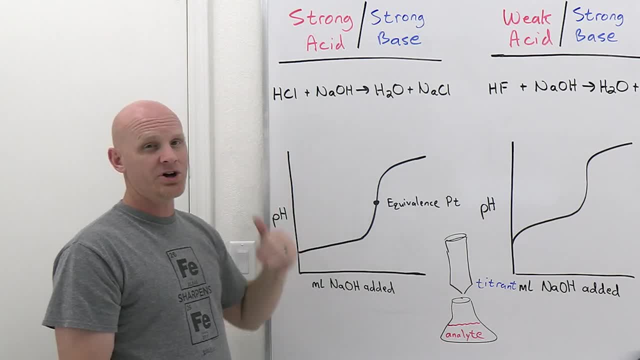 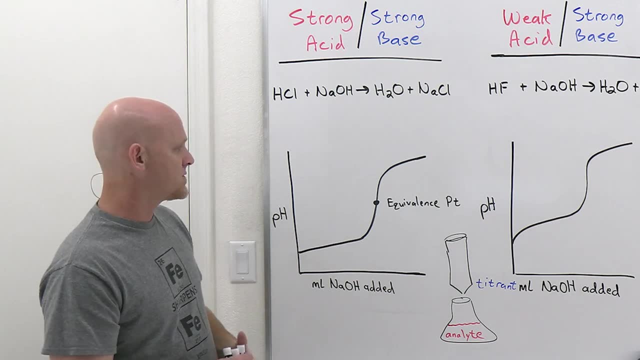 Well, in our example, HCL and NaOH react in a one to one ratio, And so a chemically equivalent amount just means an equal number of moles and a molar amount of NaOH to our HCl. So that's going to be true at the equivalence point. 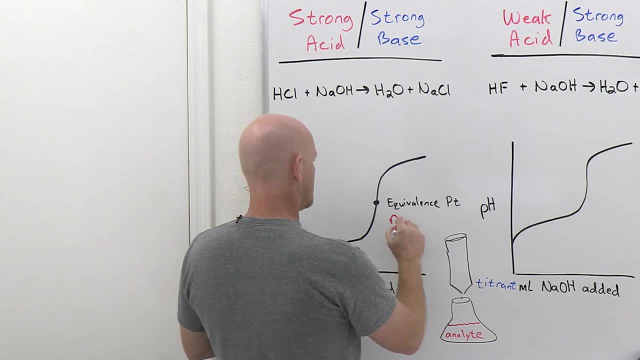 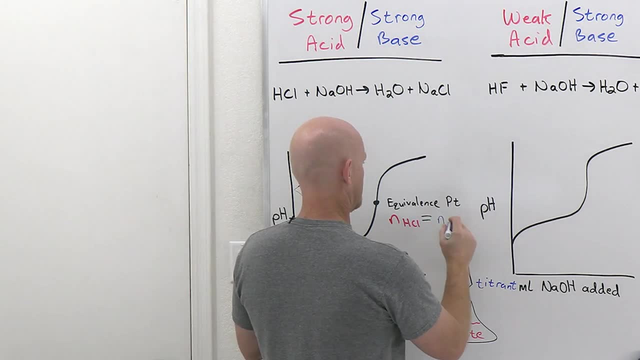 And so what that means, then, is that, at that equivalence point, the moles of HCl are going to be equal to the moles of NaOH. That's going to be true right at that equivalence point, and only at that equivalence point. Cool, And that's going to be really convenient, because 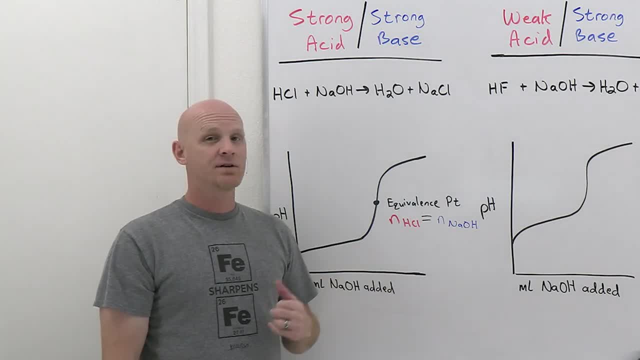 again, we're going to know the molarity of our NaOH, exactly of our titrant, And we'll be able to figure out: well, what volume of that did we add to get to that equivalence point. And once we know the molarity and volume, we can use that to find the moles of NaOH. 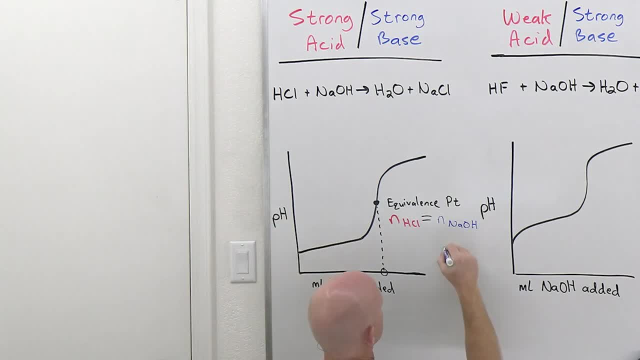 In fact, another way to write this would be to write the molarity of NaOH times the volume of NaOH, because molarity times liters is moles. And on the other side of this equation you could write the molarity of the HCl times the volume of the HCl. And now we've kind. 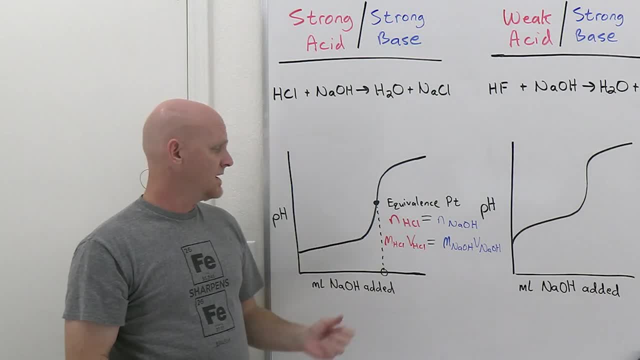 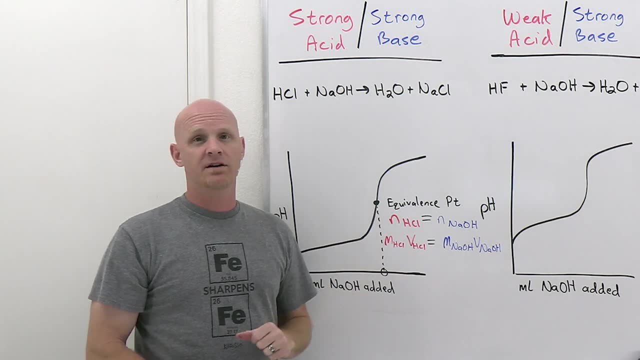 of made a really convenient equation for what's true at this equivalence point. So, because the truth is, you get to, you know, determine how much HCl you start with. You put it in that Erlenmeyer flask. If you want to start with 10 milliliters, great, Then you start. 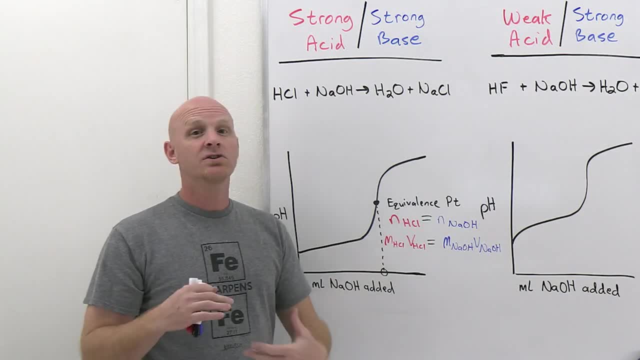 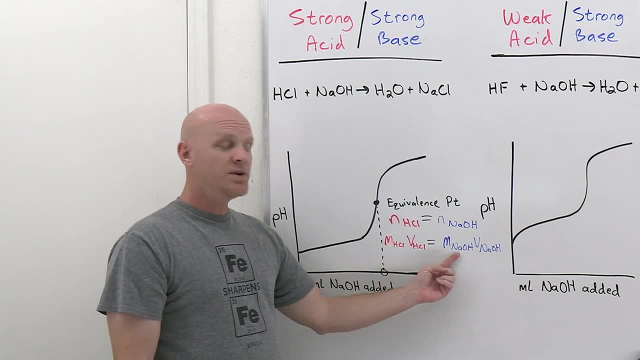 with 10 milliliters. You want to start with 50 milliliters? Great, Start with 50 milliliters. It is your choice. Whoever's you know running the titration gets to choose what that volume of HCl is going to be. Now the molarity of the NaOH is known. 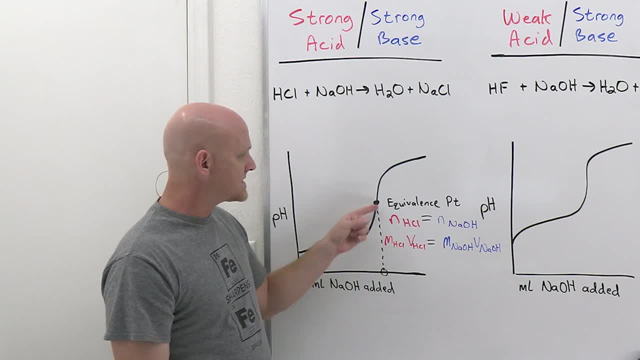 and we'll just measure with that burette how much NaOH it took to get to this equivalence point. So we'll know that volume as well. And if we know the volume of HCl we start with and then the molarity and volume of the NaOH, then we can solve for that molarity of the HCl. 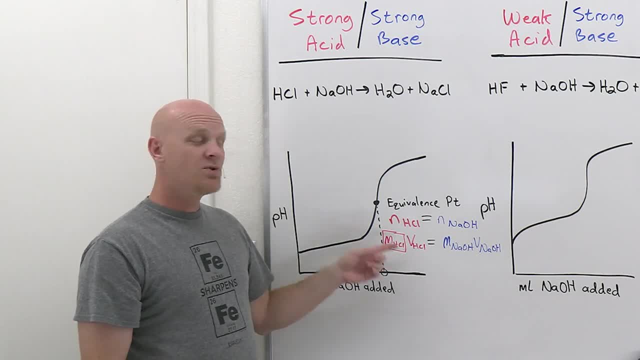 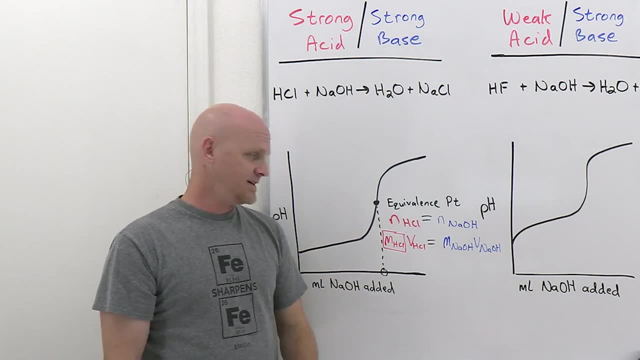 And again, that's often the point of a titration. Again, this is only true at that equivalence point. Oftentimes, the entire point of running a titration is to get that equivalence point. so we of the analyte, So how do you know if you reach that equivalence point? Well, if you're mapping, 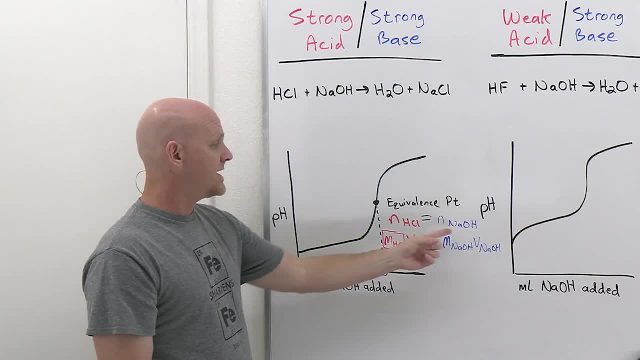 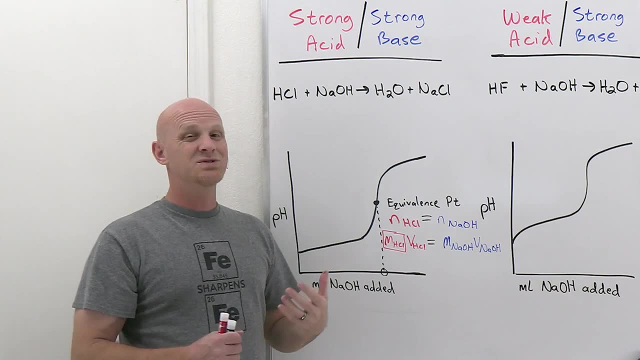 it out the entire time. you know, and you're adding a little bit of a NaOH and then taking a pH reading and you know, mapping out this curve. well then, you could figure that out, But that's not usually what we do. Normally, what we do is we use what's called an indicator. 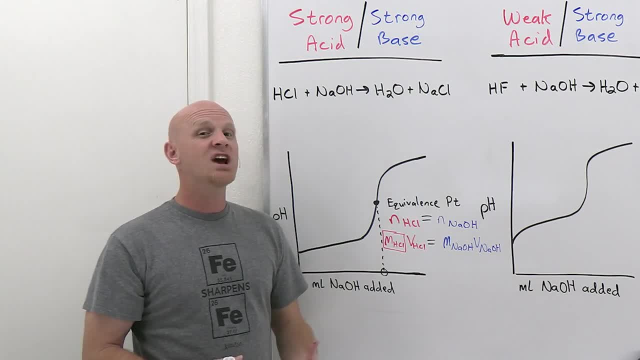 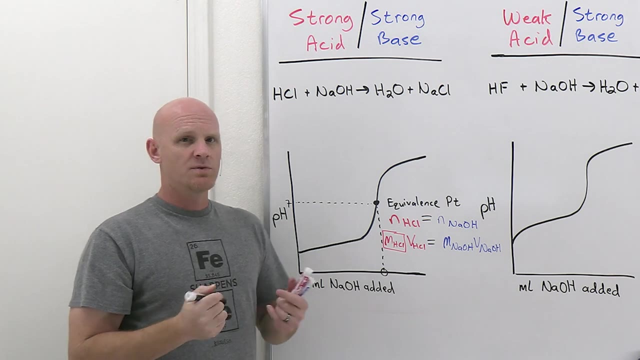 to kind of figure this out. So in an indicator is something that is going to change colors over a certain pH range, And so it turns out this equivalence point is going to occur right at pH 7.. In a strong acid, strong base titration. So we'll find out here that you know. let's say we 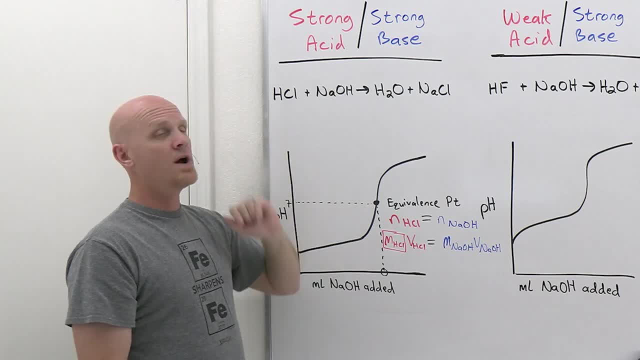 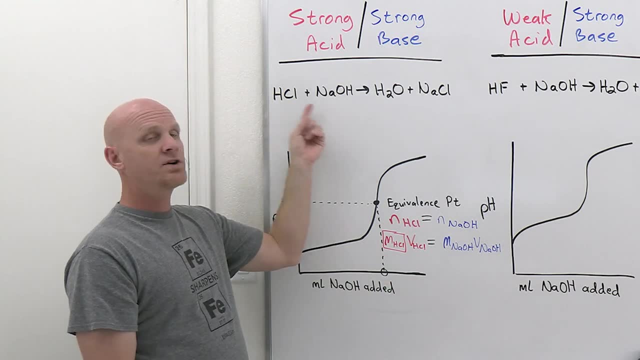 start off with 10 moles of HCl. Well, how many moles of NaOH would it take to reach the equivalence point? Well, again, the equivalence point is when we've added a chemically equivalent amount. And since, again, they react in a one-to-one ratio, then it would be an equal number of moles. 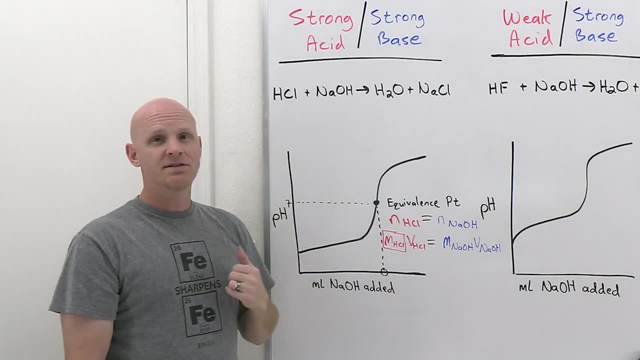 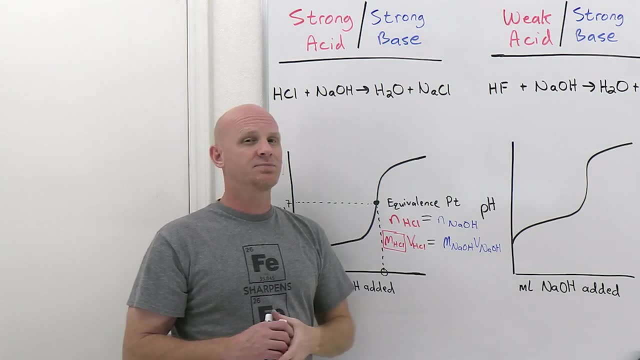 So if you start out with 10 moles of HCl, then you're going to add 10 moles of NaOH Now, because these are both strong, this reaction goes to completion. Reaction that goes to completion. you really want to look at this from like a limiting reagent. 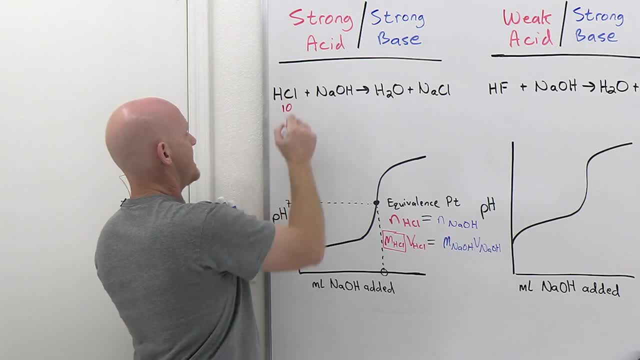 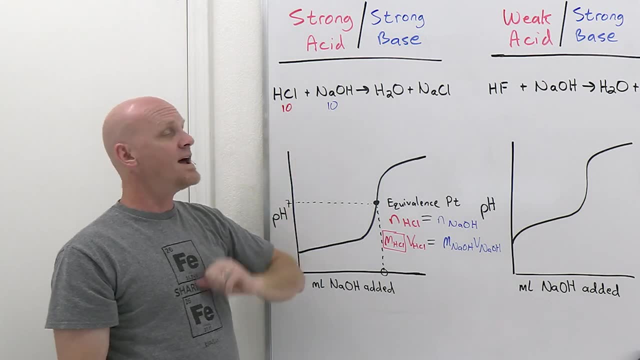 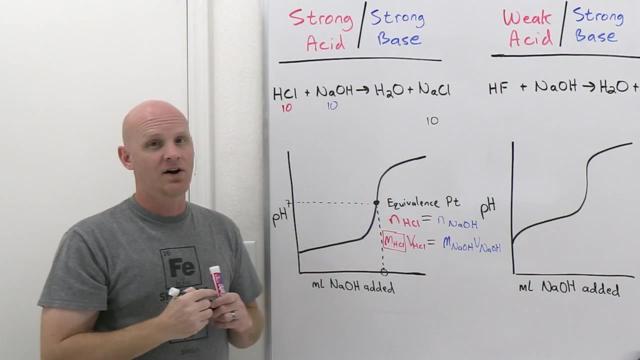 perspective. And so 10 moles of our acid and 10 moles of our base. they're going to react completely And you're not going to have any HCl or NaOH left over whatsoever, But what you will form in the end is 10 moles of NaCl. Now you'll also form 10 moles of water, but the whole thing's 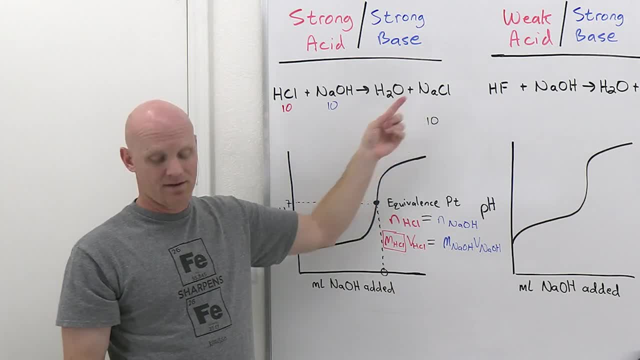 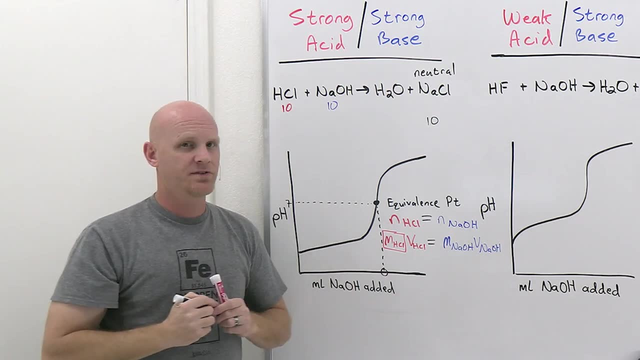 an aqueous solution, So we don't really care about that. But you're forming 10 moles of NaCl here And the important thing to realize is that NaCl is a neutral salt. So in the last lesson in chapter 16, we looked at acidic salts and basic 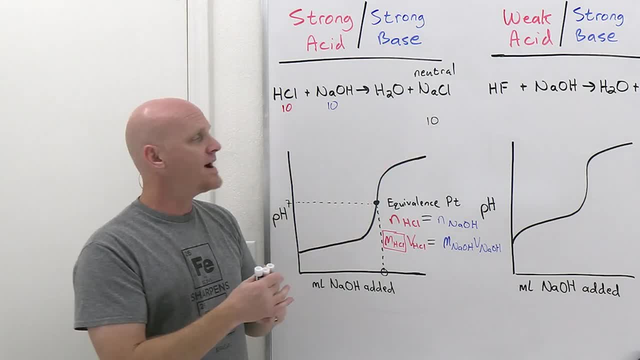 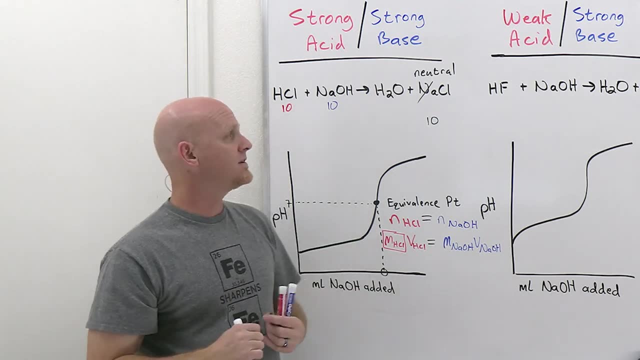 salts and neutral salts. And we learned that group 1, metal ions, and group 2, metal ions and sodiums. group 1 were negligible as Lewis acids, whereas most other cations are going to be acidic. And then we learned that the conjugate base anions of the strong acids so are the 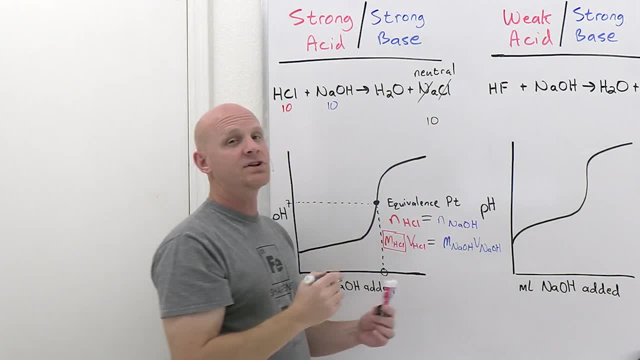 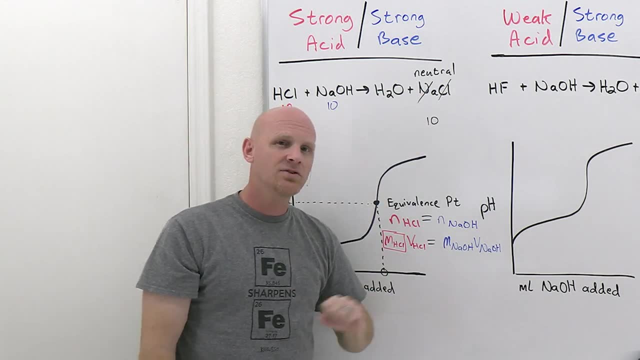 negligible anions. And HCl is a strong acid, so Cl- was a negligible anion. So in NaCl, here a negligible cation and a negligible anion was a neutral salt And that is ultimately the reason why the pH is going to be 7 at the equivalence point in a strong acid: strong base titration. 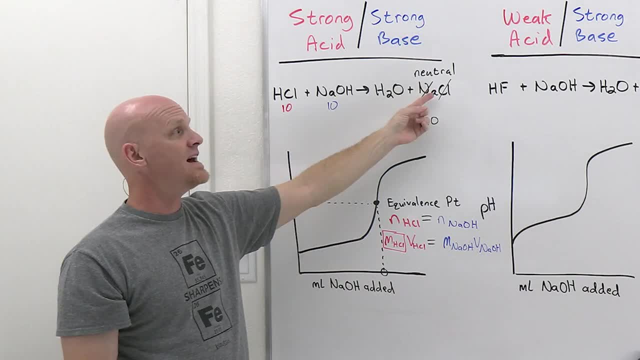 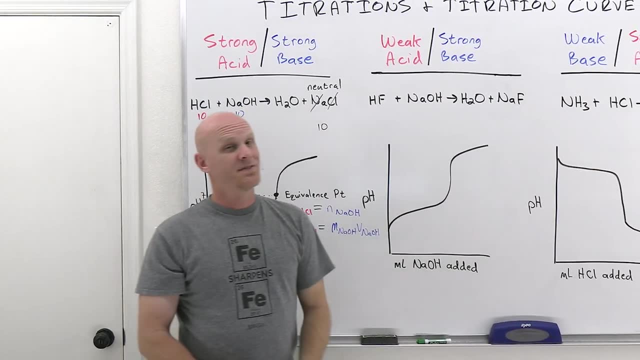 So in this case it's because the salts you produce in the titration ends up being a neutral salt. That's kind of the idea When we look at the weak acid strong base or weak base- strong acid titrations. the pH will not be 7 at the equivalence point And that's not intuitive, You might think. 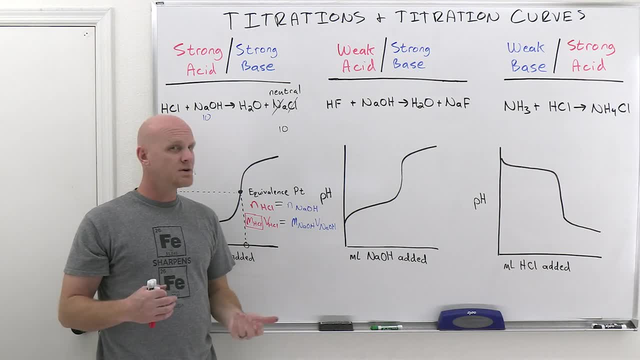 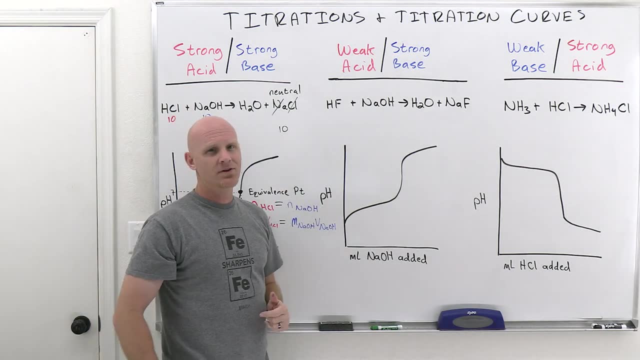 if you've added equal amounts of acid and base, shouldn't the pH be 7 and neutral? No, it turns out Now if the acid and base are both strong, yes, but not if one's weak and one is strong, And it. 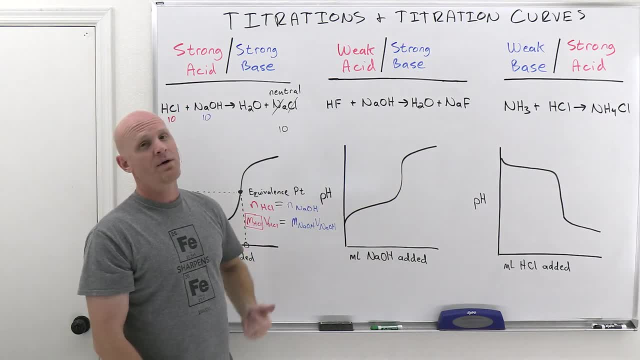 turns out. my personal way of remembering this is: I just look at whoever's strong and they win at the equivalence point. So we'll find out. with a weak acid strong base, the pH is going to be a little bit basic at the equivalence point, a little bit higher than 7, like 7 to 10.. And in a 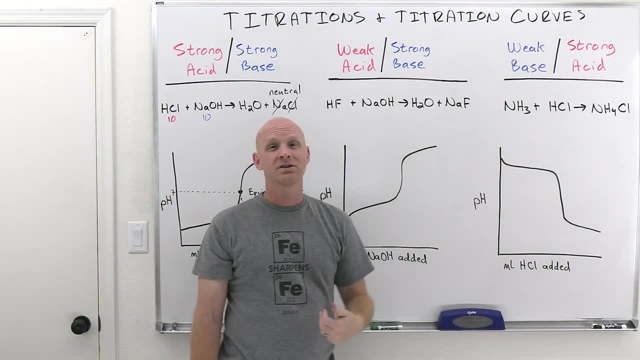 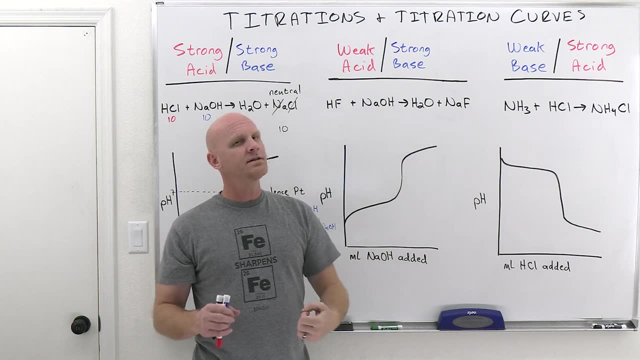 weak base. strong acid titration: it's the acid that is strong, And so the pH will be a little bit acidic at the equivalence point, probably somewhere between 4 and 7.. Now that's how I remember it, But, as we'll see, that's not really the reason why the pH is going to be so strong. 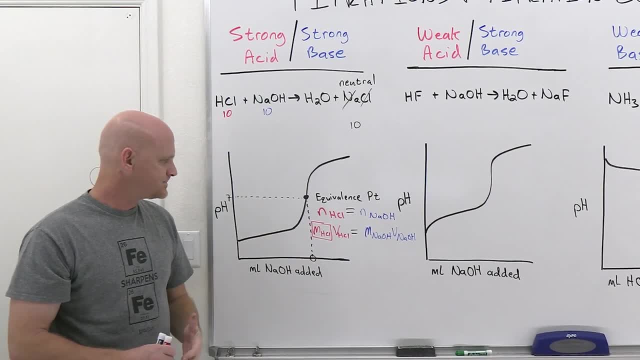 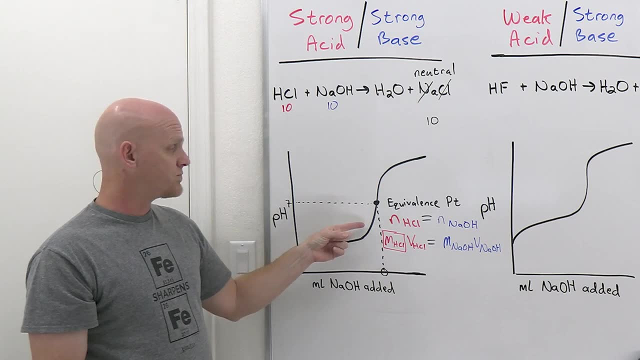 But we'll come back to that in a bit. Okay, So one more thing about our indicator here. So you want your indicator to change colors right around that equivalence point. Well, it turns out, indicators don't just change color over a small pH window, It's actually over a pretty 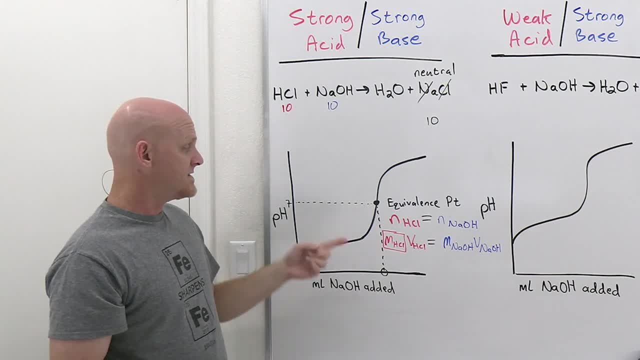 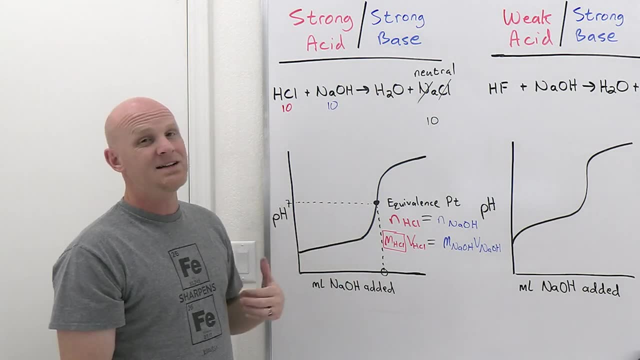 significant jump. usually a couple pH units jump. But what's nice is that you know your pH jumps very quickly right across that equivalence point. So again, from down here to somewhere up here it's usually only a difference of a drop or two. 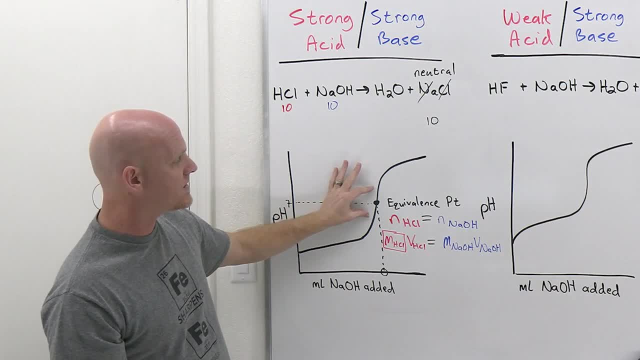 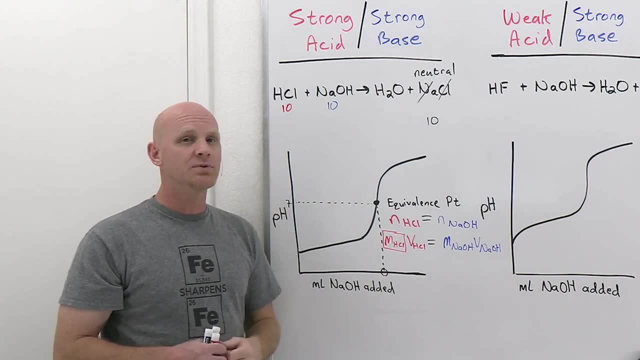 And so you want to choose an indicator if it's going to change color right across that window in the 6 to 8 range, maybe in this particular titration. So, and it turns out phenolphthalein is a really common example of a good indicator to use in a strong acid, strong base titration. 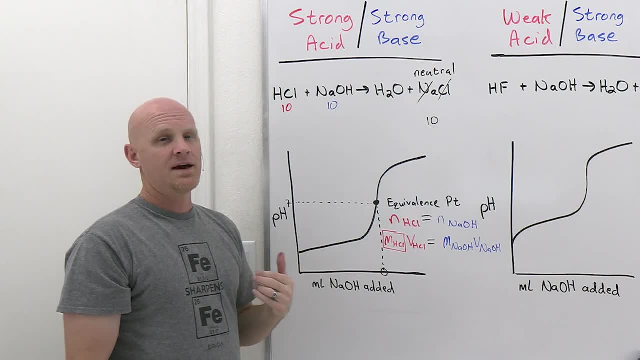 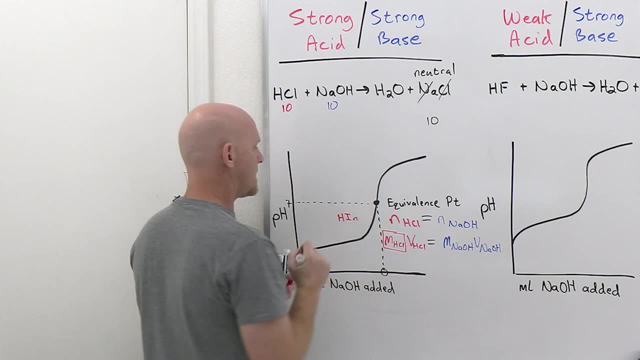 because it will change colors right across that window. And it turns out that phenolphthalein itself is- I'll just abbreviate it as an indicator here- it itself is an acid, a weak acid, So it has a weak acid. 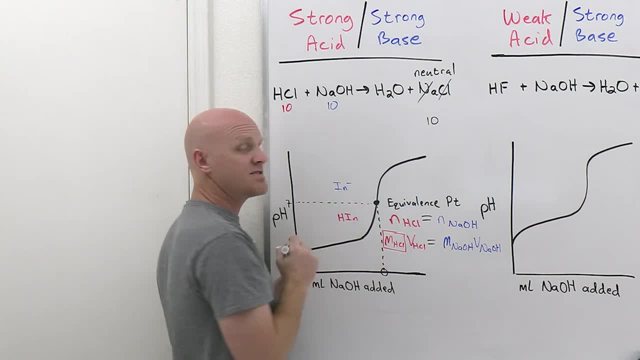 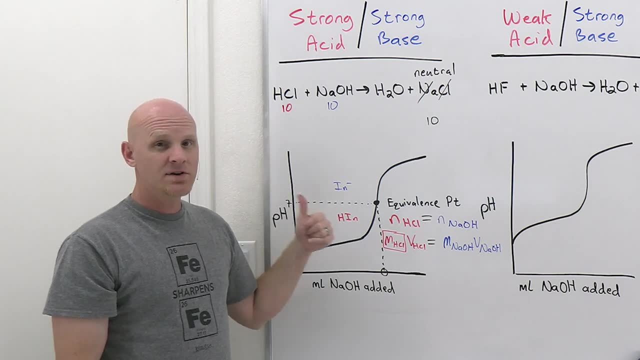 And it has a conjugate base form which I'll just represent this way. It's actually a rather large molecule that I'm not going to draw it or anything like that, So, but I'll represent it in these two forms here. And it turns out so that as you add NaOH, it itself also gets titrated, And so it. 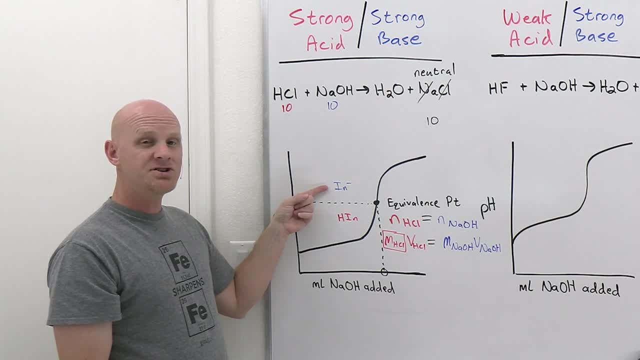 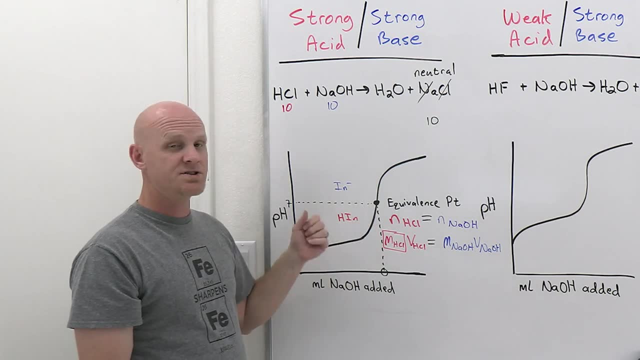 turns out. in its acid form, it's colorless. In its conjugate base form, though, it has a pinkish, purplish color, And so, as you blow through this equivalence point again over the course of just like an extra drop or two of NaOH, the solution goes from there, And so you can see that it's. 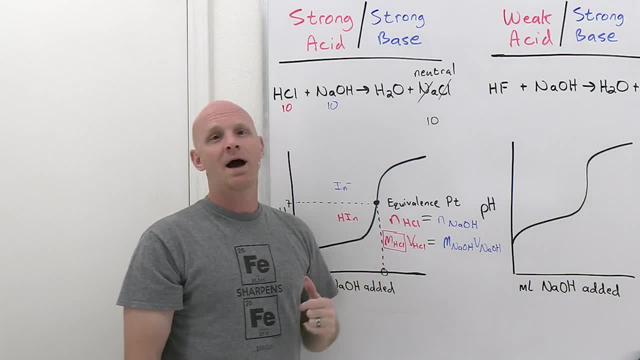 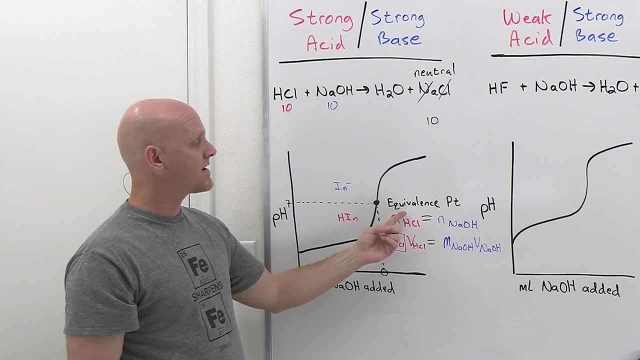 from being colorless to being pinkish, purplish, And once that happens, you know you've reached the end of your titration. So, and you've reached what's called the end point, And your end point is your best approximation of that equivalence point. So these color change indicators are, by 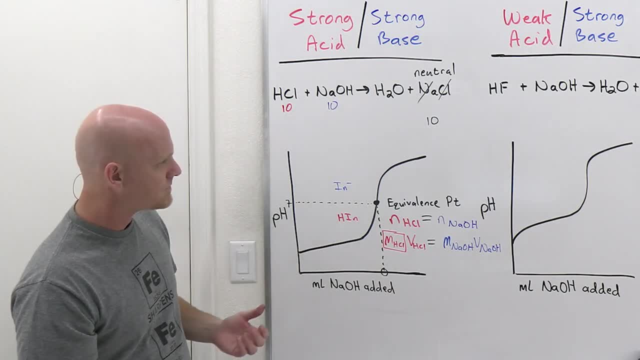 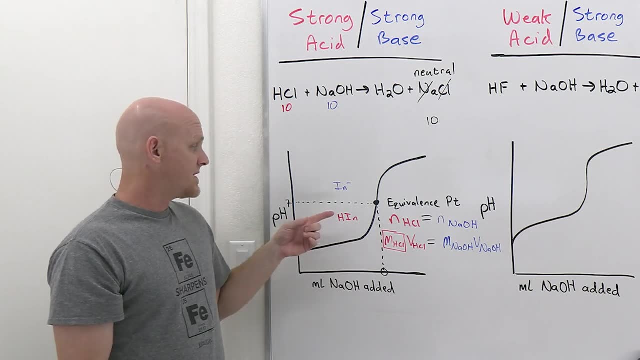 far the most common example of an indicator you're likely to see. Okay, So it turns out. then, if you know, we learned this with buffers in the last lesson. So when you've got a weak acid conjugate base, well, it turns out. if the pH equals the pKa of 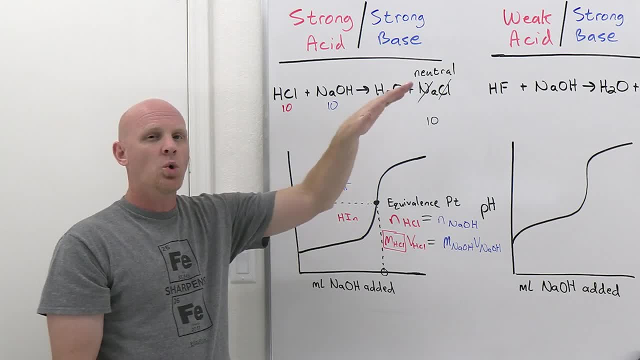 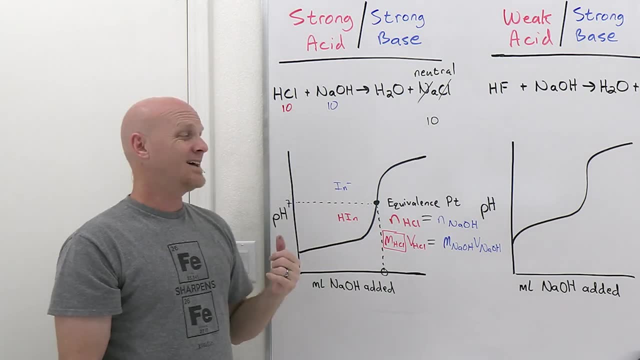 then these will be present in equal concentrations. But if you go one pH unit lower than that, you'll have 10 times more acid. One pH unit higher than that, you'll have 10 times more conjugate base. And so in this case, if we want the pH in our titration to turn colors, change colors. 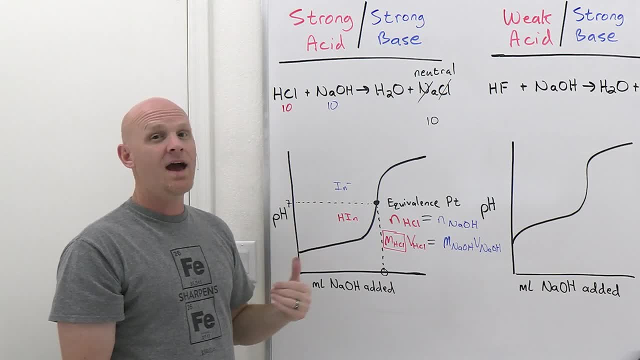 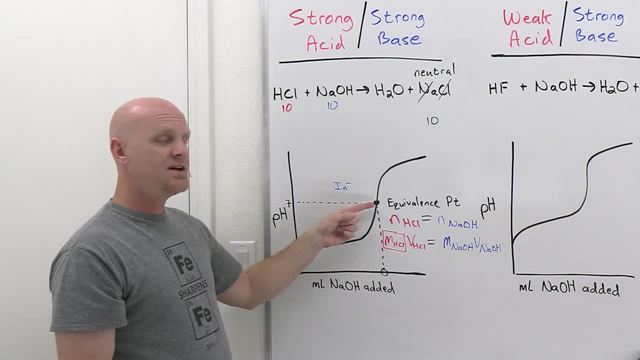 right around pH 7,. well then, the indicator should have a pKa right around 7.. So cool. So you want your indicator to have a pKa right around whatever pH you have at the equivalence point. Cool, And it turns out we've got a whole slew of different indicators And the thing is that 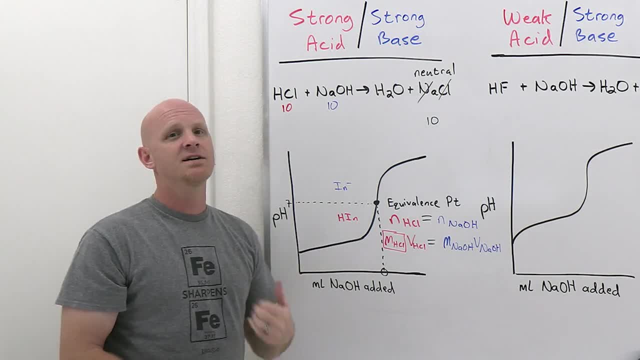 they're at least brightly colored in one of the two different versions so that we can use them, like is in the case with phenolphthalein, where it's brightly colored in the base form but colorless in the acid form. Some change from like red to green and things of the sort. So 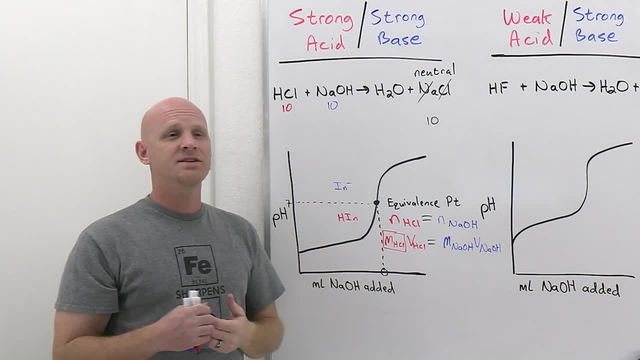 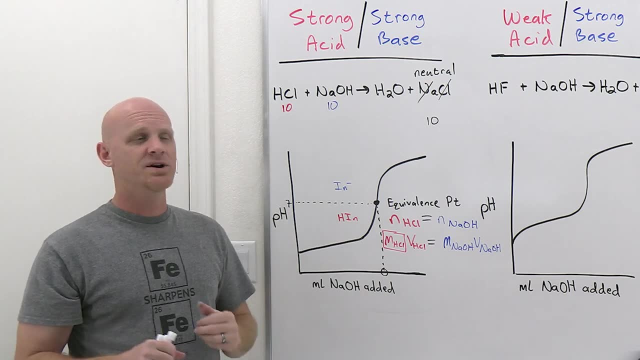 but we have a whole host of them And we have we discovered over time, and they change colors at different pH ranges And so we can kind of look up in a table what their pKa's are and choose the appropriate indicator for whatever titration we're doing. 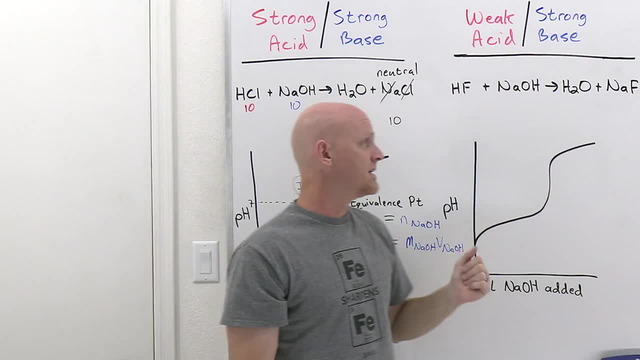 Okay, So we've got a whole slew of different indicators And the thing is that they're at. Let's take a look at our weak acid, strong base titration, And in this case, the weak acid we're going to look at is HF, and we're still going to use NaOH, And again, because NaOH is a strong 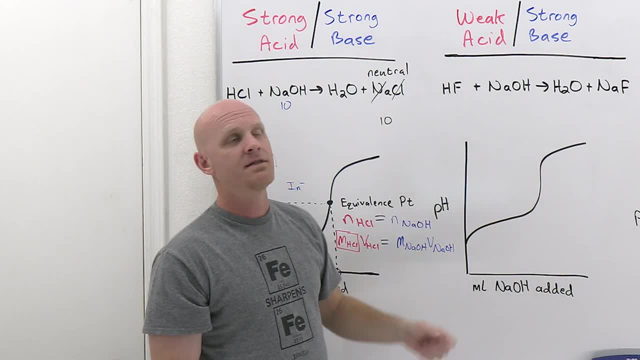 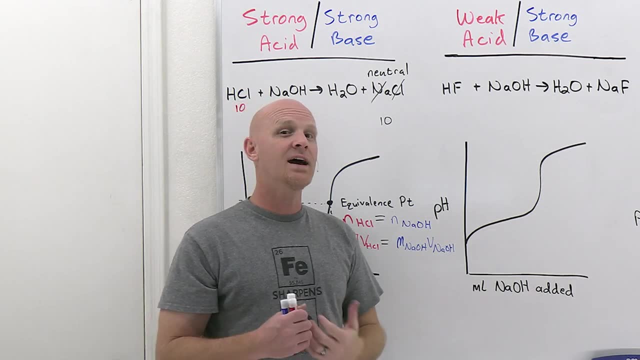 base. as long as the acid or the base is strong or both, this reaction will go 100% to completion, And so we're going to look at it as kind of a limiting reagent problem again, And we'll incorporate that into our pH calculations in the next couple of lessons. Now, big difference here. 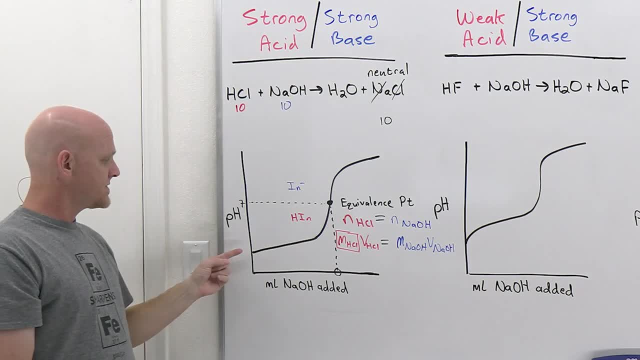 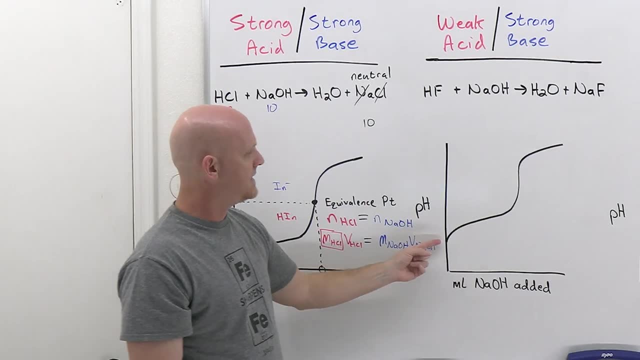 is, what you're going to find out is with a strong acid, strong base titration. So you'll find out that when you first start the titration you're adding NaOH. you get this nice long linear region. So, but right at the beginning, in a weak, strong titration, you're going to get a big change in pH. 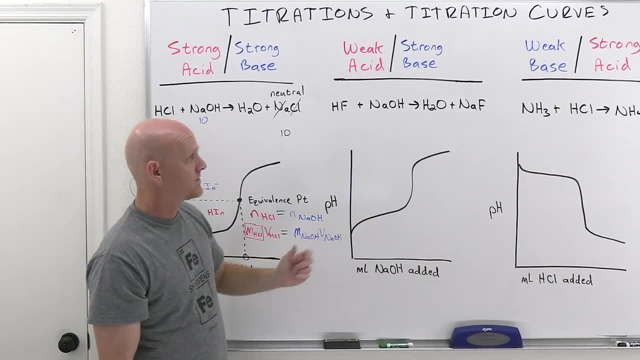 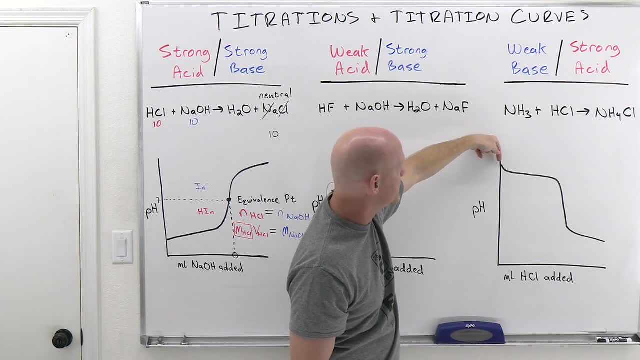 right at the beginning and before it kind of flattens out a little bit And notice we see the same thing over here with weak base, strong acid. In this case we're starting out with the base and adding the acid, So the pH is going to go down, so you get a real sudden pH drop right at the 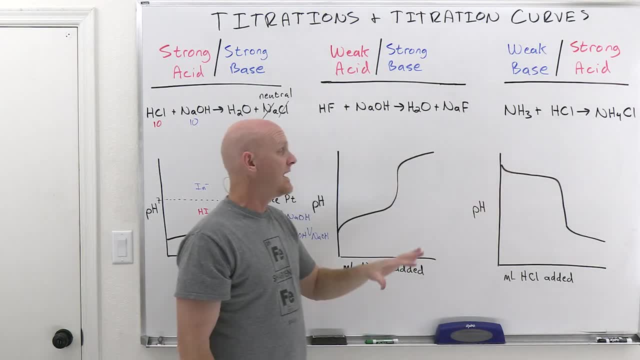 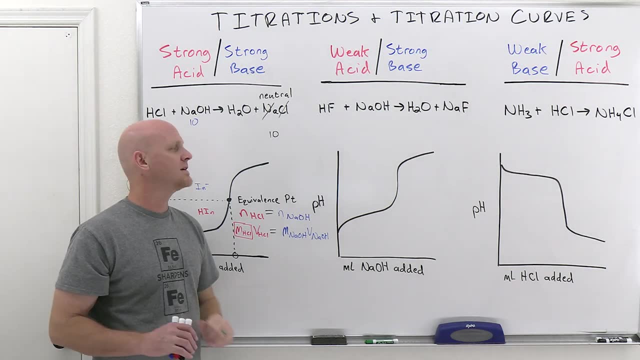 initial point before it kind of flattens out a little bit and goes linear, And so that's characteristic if you've got a weak strong titration versus a strong acid, strong base strong titration, One of the key differences you can tell, but it's kind of a minor point. 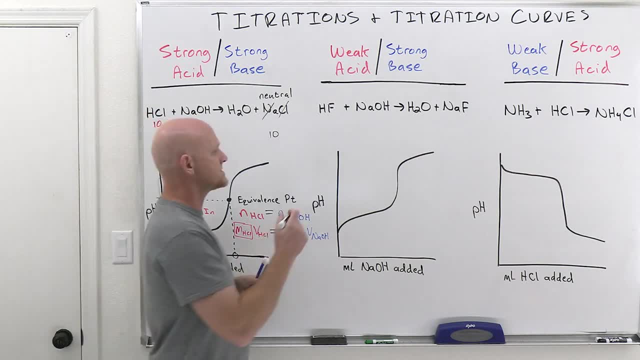 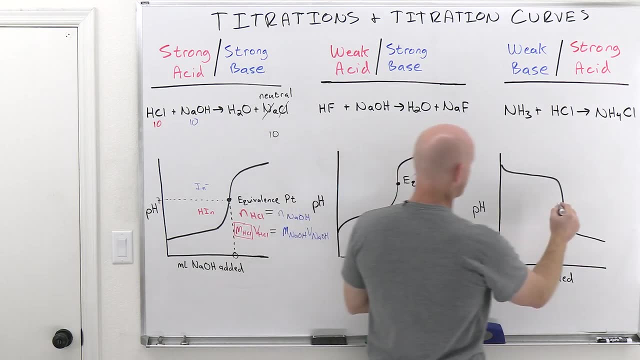 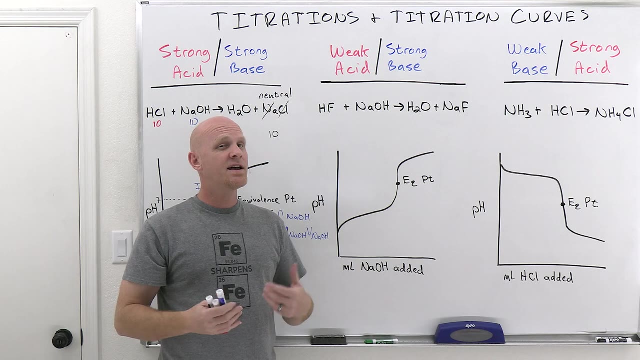 as we'll point out here in a second, because that'll be an easier way to tell Now, you're still going to have an equivalence point here. That's the inflection point in both of these. here, it turns out, And that equivalence point is still when you've added a chemically equivalent amount of titrant. 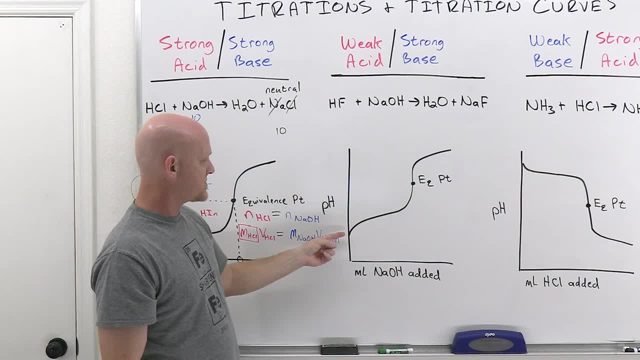 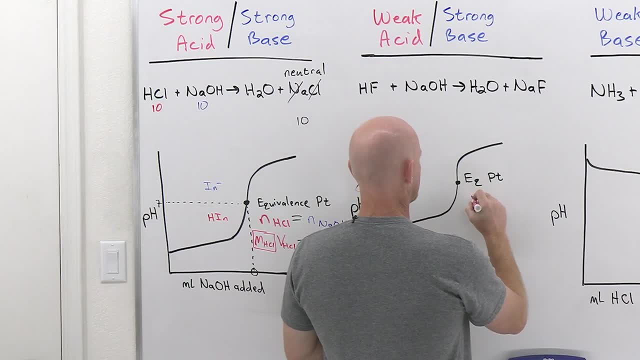 to your analyte, And in this case our analyte is the HF. We're starting off with an acidic solution and the titrant is the NaOH, And so at that equivalence point you're going to have the moles of HF equal to- let's put that in black- the moles of NaOH, in this case. 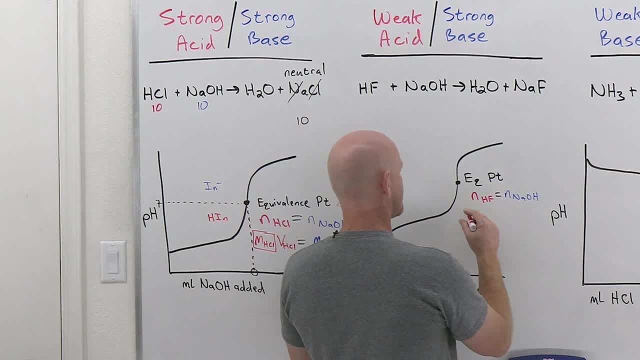 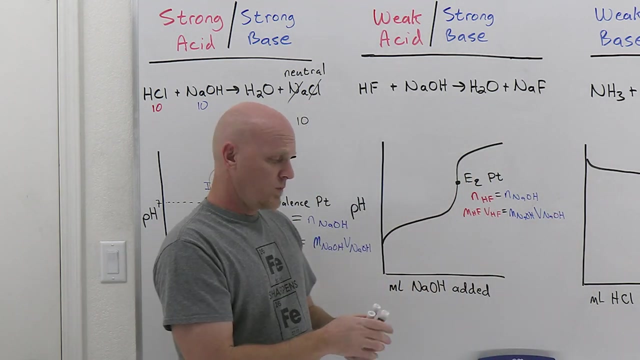 And what that means. again, we could write that in a more convenient form. We could say that the molarity of the HF times the volume of the HF is equal to same thing for the NaOH. Cool, And once again you're going to know the molarity of your NaOH. You could figure out what. 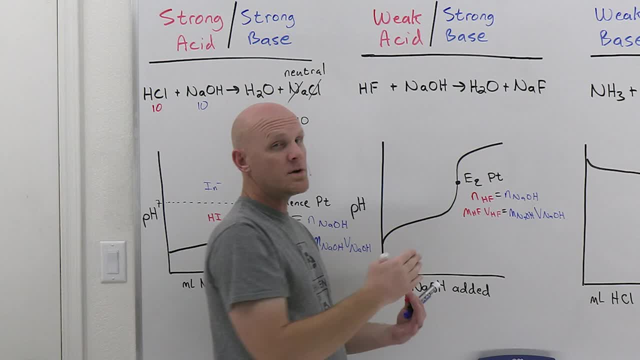 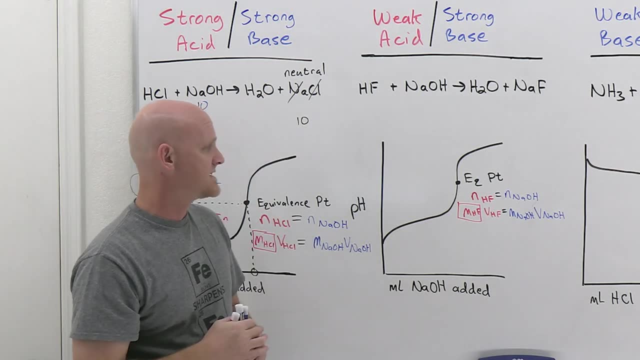 volume it took to get to the equivalence point. You get to choose what volume of HF you start with, And so you can use that to figure out what volume of HF you start with, And so you can use that to solve for the molarity of your analyte the HF in this particular example. 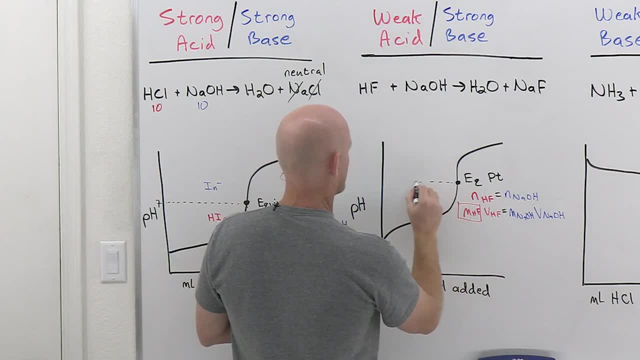 Cool, Now. what you will find out, though- if we kind of drag this across, though- is that, again, your pH is not going to be 7 at the equivalence point. You're going to find out that it's going. 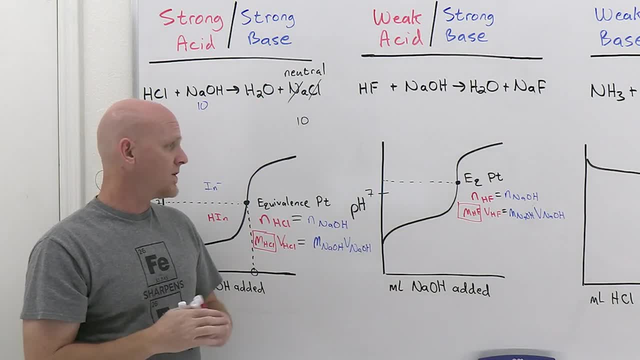 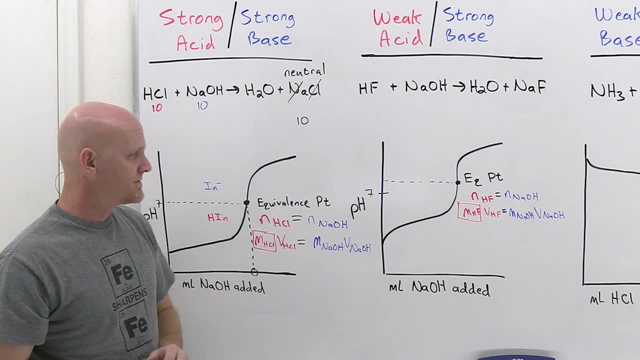 to be higher than 7.. So, and again, usually not super higher than 7, but somewhere probably in the 7 to 10 range, depending on you know what exact weak acid you've chosen and things of that sort and what concentration it has. So both play in a factor, But the key is the pH is going to be. 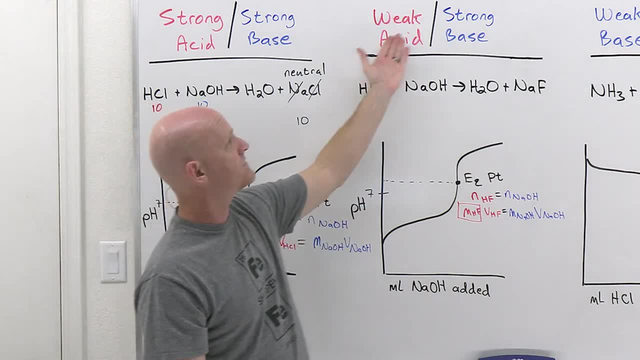 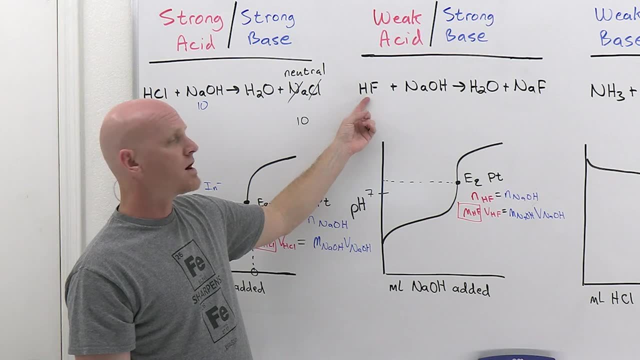 a little bit basic. Now, again, my way of remembering this is: I look at weak acid, strong base. The base is strong and it wins at the equivalence point. But again, that's not really the reason. The reason, so notice, if you start off with 10 moles of HF and you add 10 moles of NaOH. 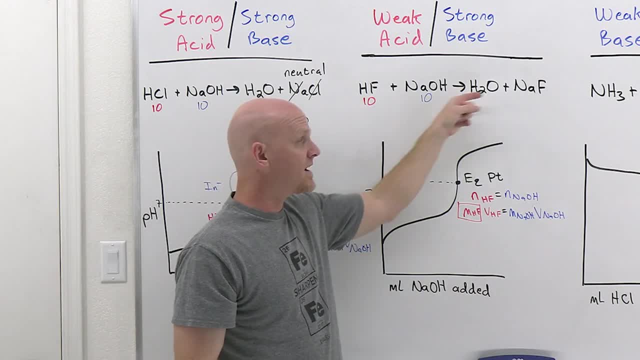 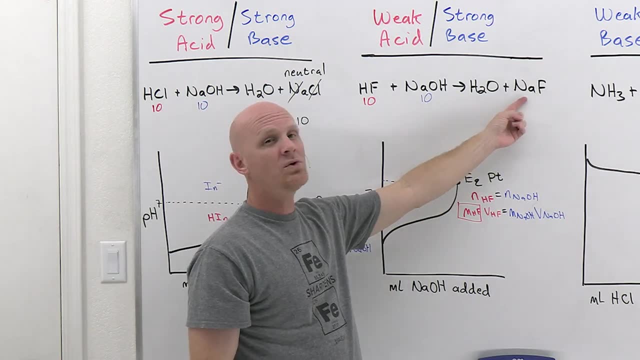 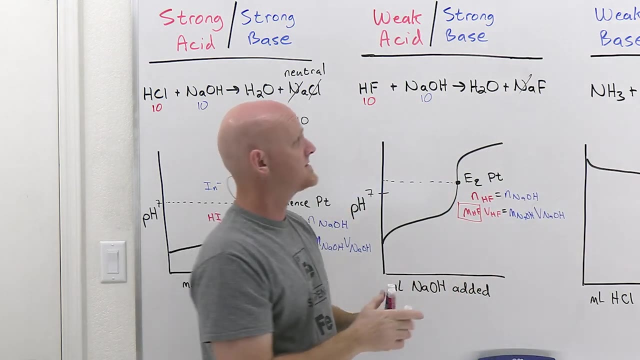 so they're going to react completely and, you know, going to neutralize each other completely so that you have no HF and no NaOH left whatsoever. But in this case you're going to form 10 moles of sodium fluoride And whereas, again, sodium, being group one, is still negligible, the fluoride is not. So the 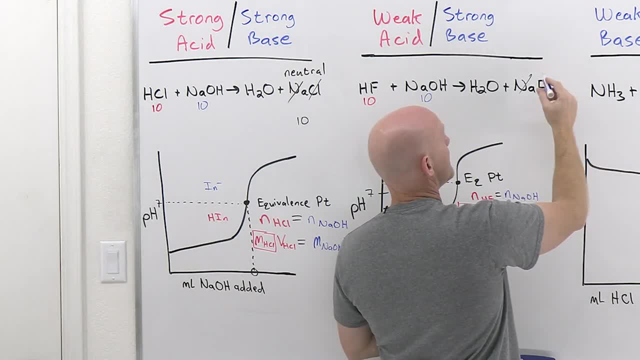 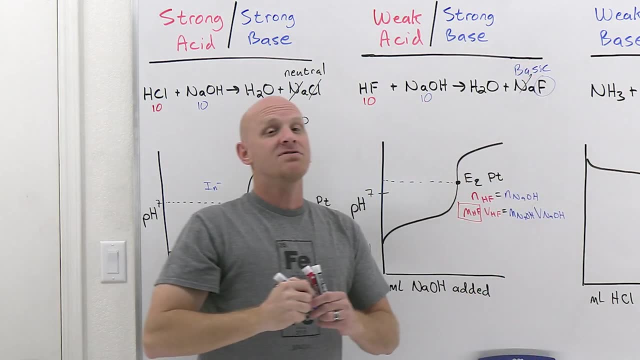 fluoride is not the conjugate acid of- I'm sorry, not the conjugate base of- a strong acid, but the conjugate base of a weak acid, and is therefore really a base, And so this is a basic salt, And that is ultimately the reason why the pH is going to be basic. It's because the salt that you produce 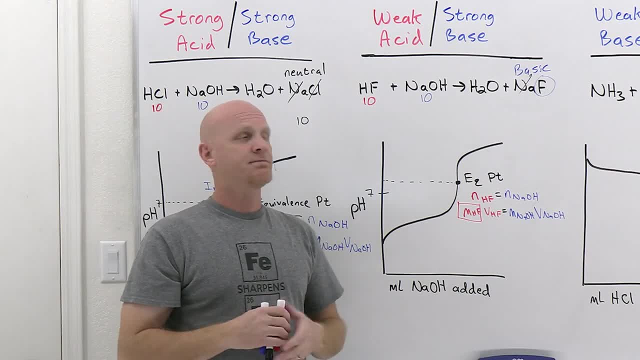 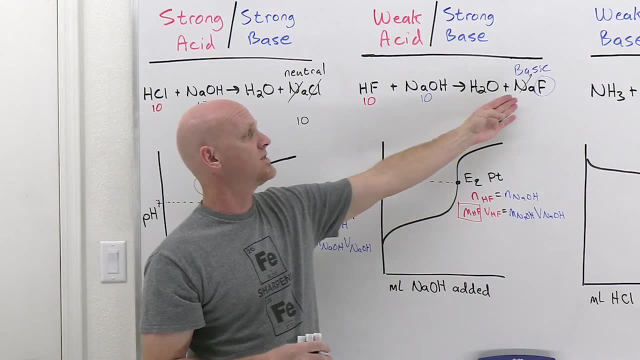 is a basic salt. Now, if they, just you know, if I asked you why is the pH greater than 7 in a weak acid strong base titration, The equivalence point? So if you said because the salt that is produced is a basic salt, that is 100%. 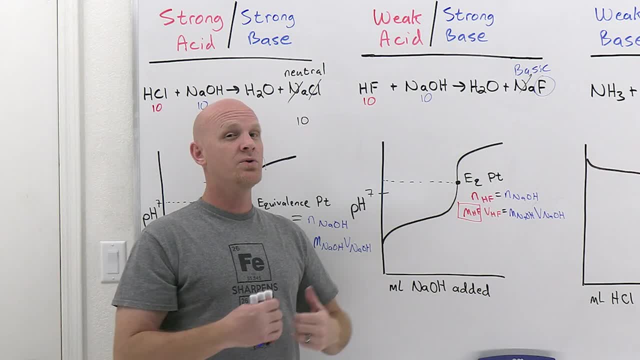 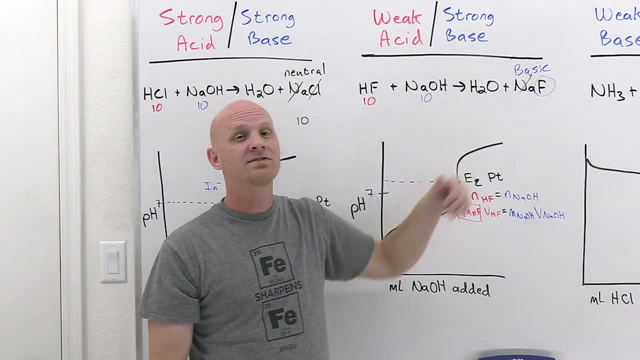 true. So but if you had to choose, kind of like, which of the following is true on a multiple choice test, they might phrase it that way, but they might phrase it a little bit different. So instead of saying that sodium fluoride is a basic salt, they might say that it undergoes hydrolysis. Let me put 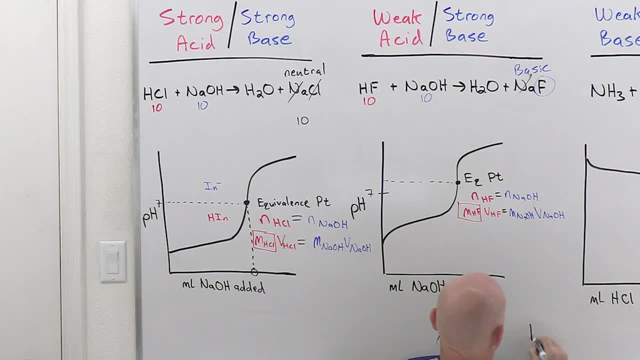 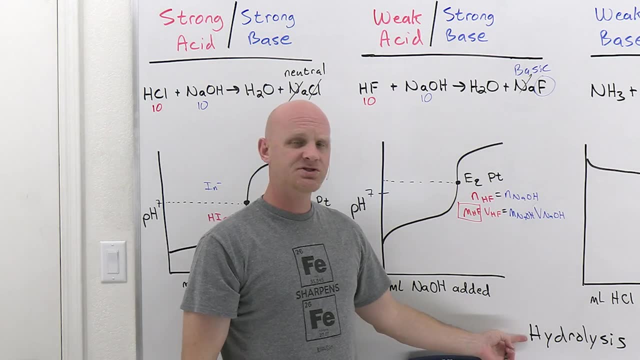 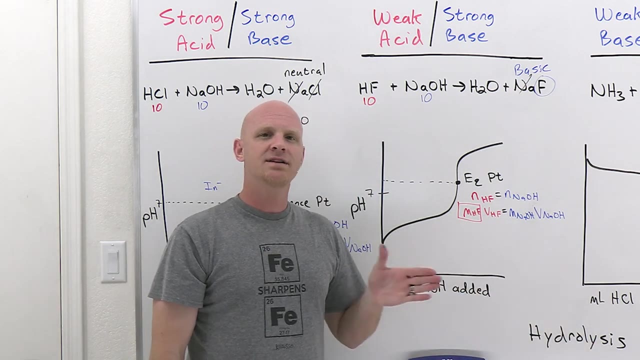 that word up on the board here somewhere, If you look at that word: hydrolysis. hydro refers to water, lysis means the splitting or destruction of. So this is the destruction or splitting of water. Well, it turns out that any chemical reaction that has water as a reactant 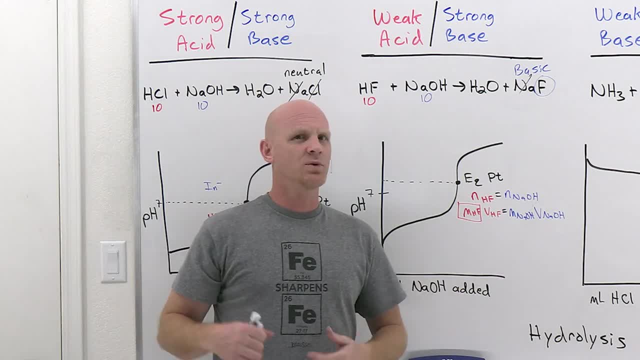 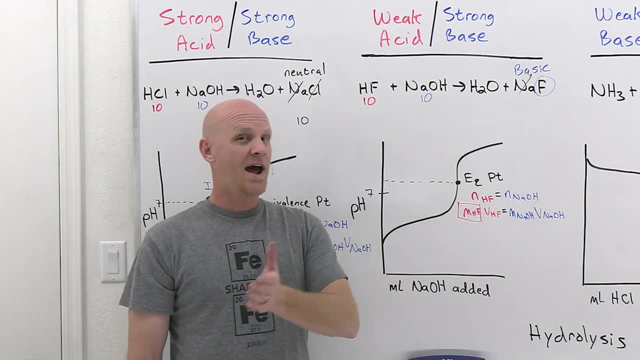 where water gets used up. kind of water is getting destroyed, if you will. it's getting used up, it's getting consumed, And they call it a hydrolysis reaction. Well, an acid base reaction that reacts with water, where either an acid reacts with water to produce hydronium or a base. 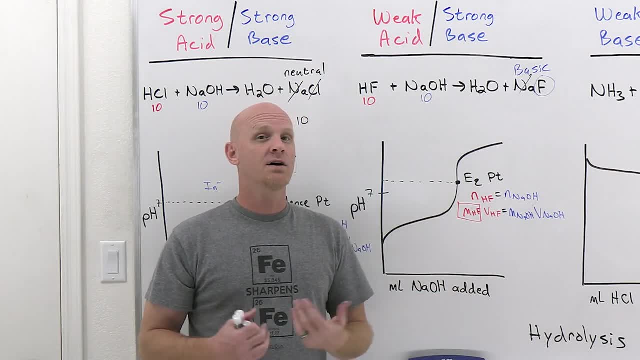 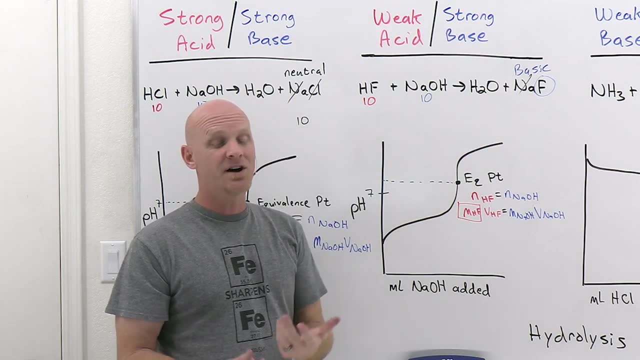 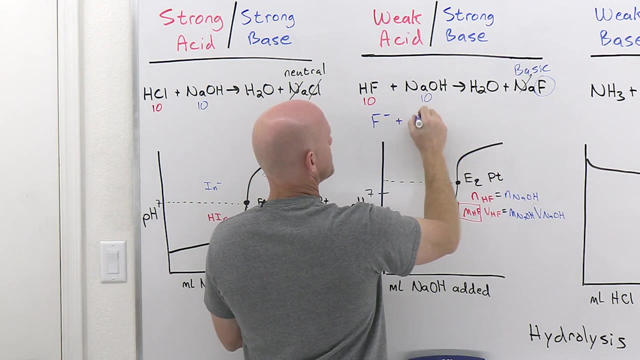 reacts with water to produce hydroxide. Those are examples of hydrolysis reactions. Sometimes we call them acid hydrolysis reactions. sk, Chelsea, calm, This is gonna undergo base hydrolysis And so, in this case, your F minus that you produced, right. 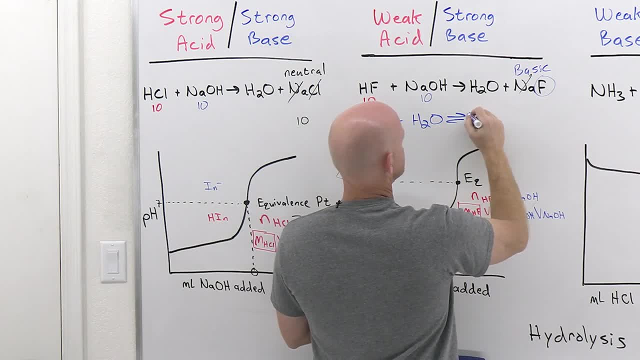 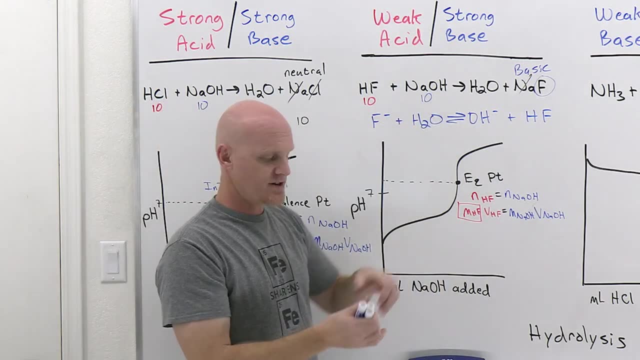 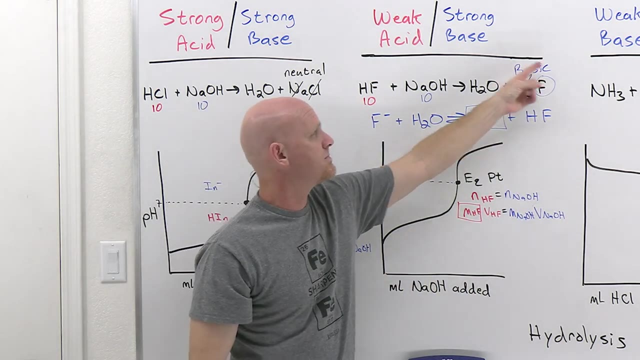 here is then going to react with water to produce some OH minus and some HF, And so this is the hydrolysis reaction. This is why the solution is basic at the equivalence point, because the fluoride sodium, fluoride salt- that's basic- reacts with water to produce some fluoride. Notice it also. 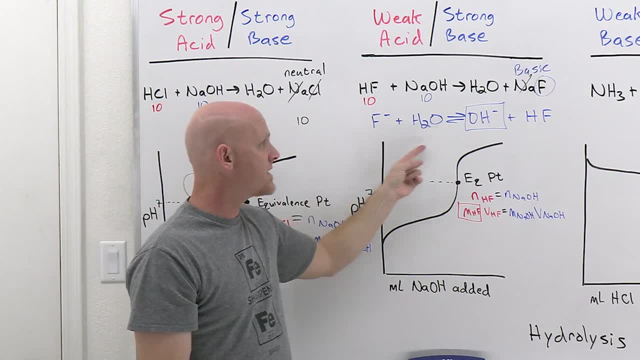 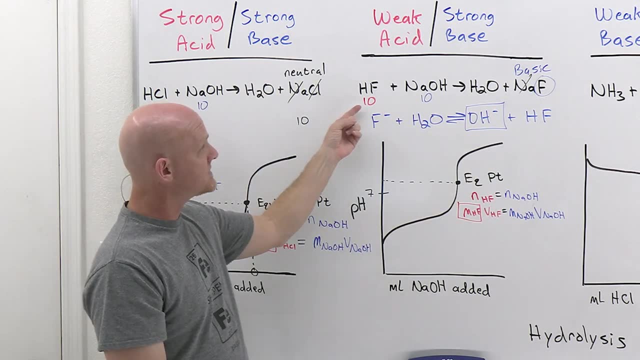 implies that you actually don't end up with zero HF, because the fluoride, when it undergoes hydrolysis, produces a tiny amount in this equilibrium. The solution, technically, is not going to have zero HF. It initially looked like it was going to, but you will have a super tiny. 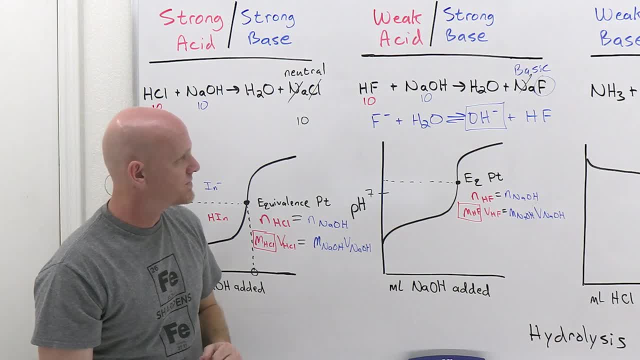 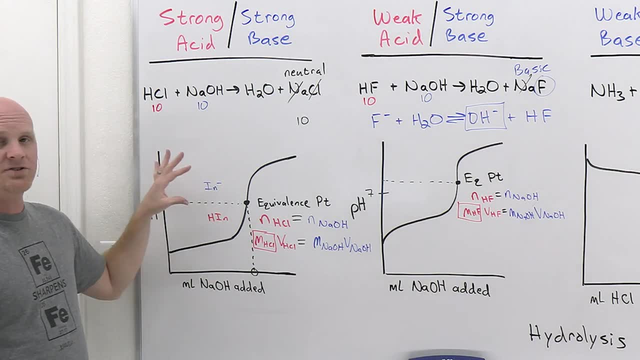 amount, in this case an amount that's equal to the amount of hydroxide you produce. Cool, Now we've got something else to address here, And it turns out we didn't have to worry about this on the strong acid, strong base titration, but with the weak strong titrations. 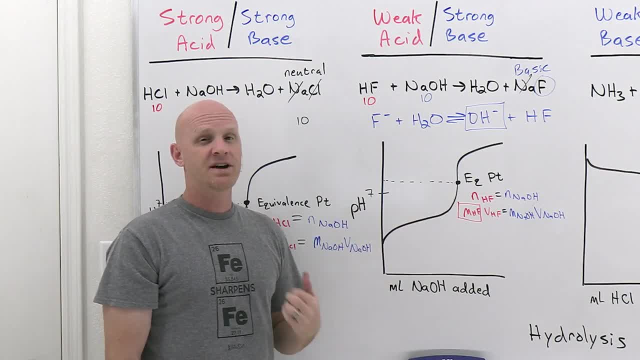 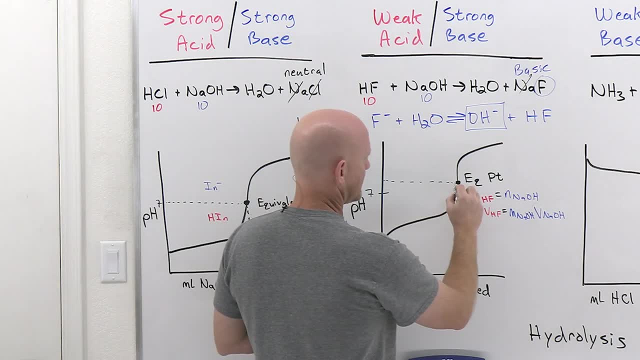 there are not just one important point, the equivalence point on the titration, they're actually going to be two important points And the other one is going to be halfway to your equivalence point. So let's say, for example, at that point right there happened at like 20. 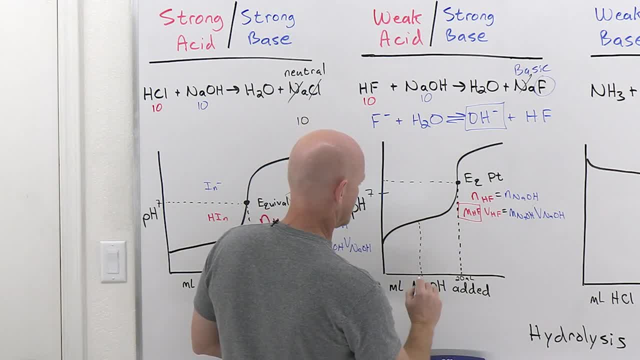 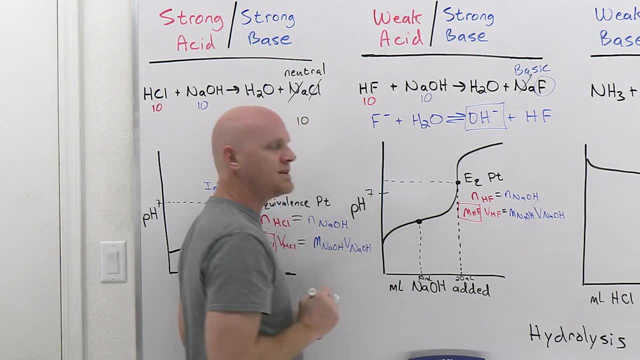 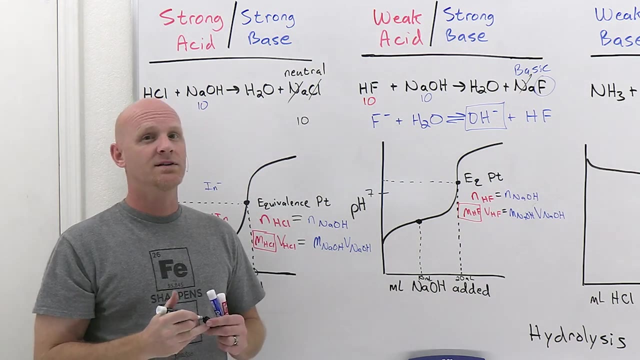 milliliters. What we'd do is we'd go back to 10 milliliters. So, and that point right here would be halfway to the equivalence point. We might call it the half equivalence point or the half neutralization point, And it is a special point, So we didn't have to worry about. 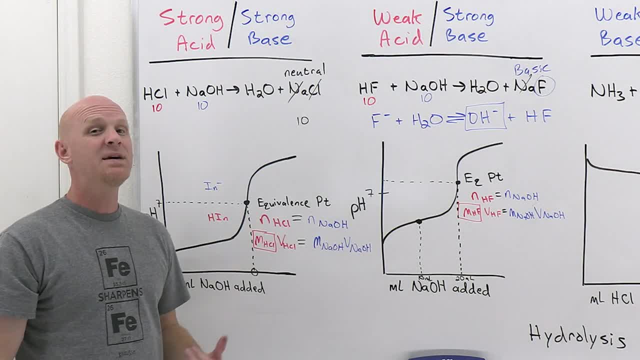 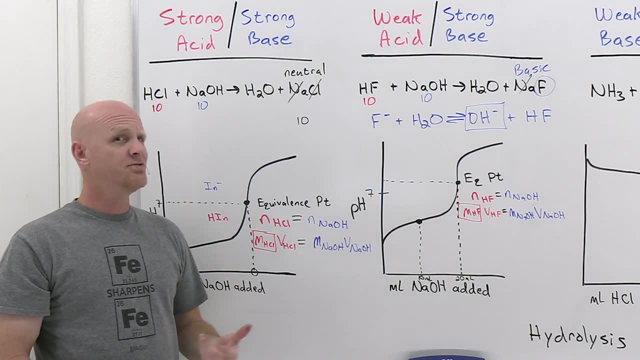 that here, as it turns out, but we're going to use this point to find the pKa of our acid. Well, for strong acids, we just say they dissociate completely. So and that implies that their KAs are infinity. Well, they're not infinity, They're just really huge numbers. So, but we never talk. 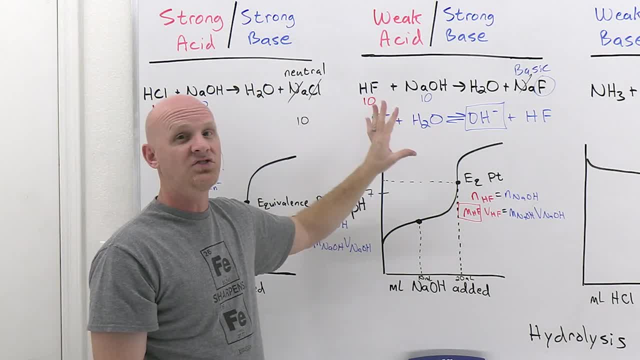 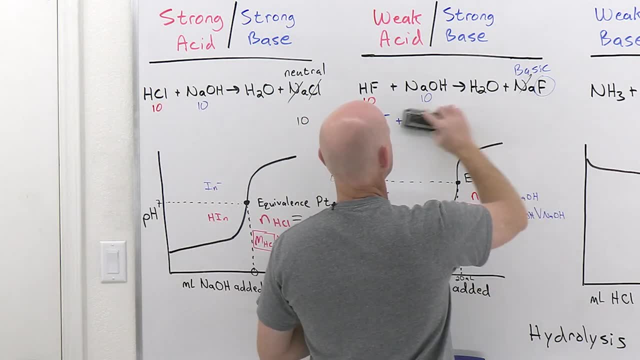 about their KAs or their pKAs. But for weak acids we do, and that's because they're not infinity, And that's why this now becomes relevant. Well, right at this half equivalence point, let's see what's true here for a second now. So if it took 10 moles of NaOH to get 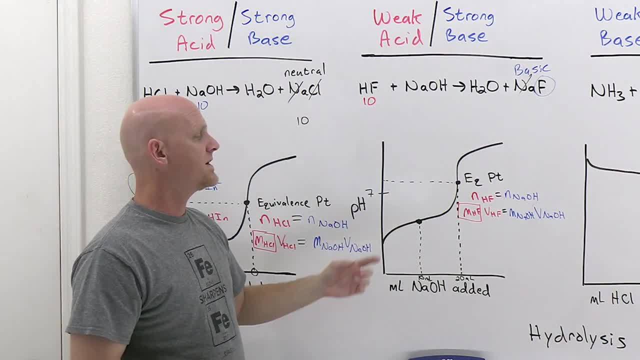 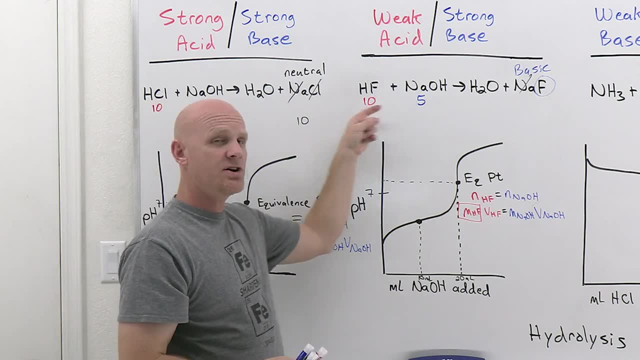 to the full equivalence point. one-to-one ratio, chemically equivalent amounts. well then, to get halfway, there would only be half as much, And in this case, again, this reaction is going to go to completion, since NaOH is a strong base and NaOH would be the limiting. 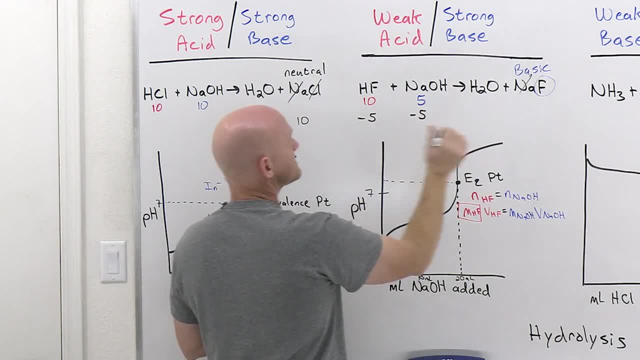 reagent And five moles of the NaOH would neutralize five moles of the HF to produce five moles of the NAF. And what you're going to find out is that you're going to have five moles of HF left in your solution, but you're also going to have five moles now of the conjugate. 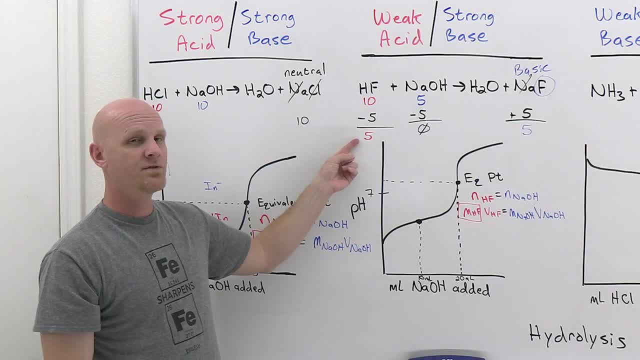 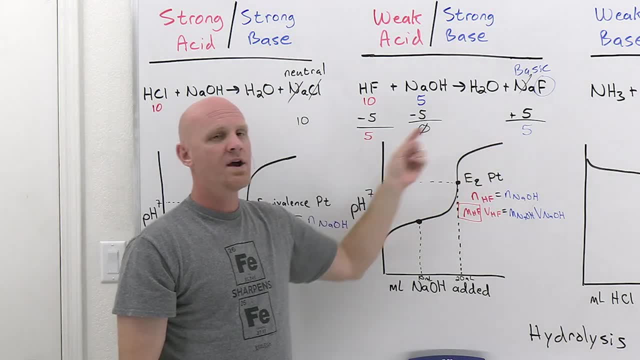 base, the F- And notice that's interesting because you have five moles of a weak acid and five moles of its conjugate base. And you guys learned in the last lesson that when you have close to one-to-one ratio of a weak acid and its conjugate base, you have a buffer. And notice how 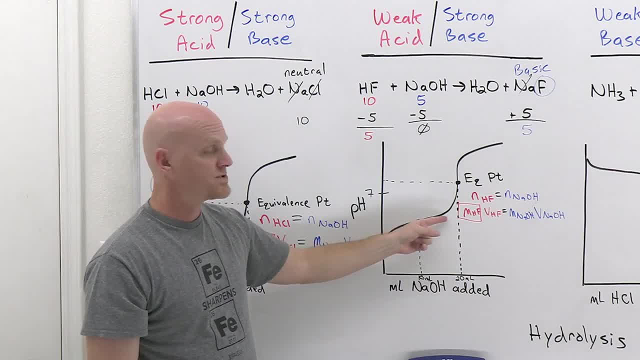 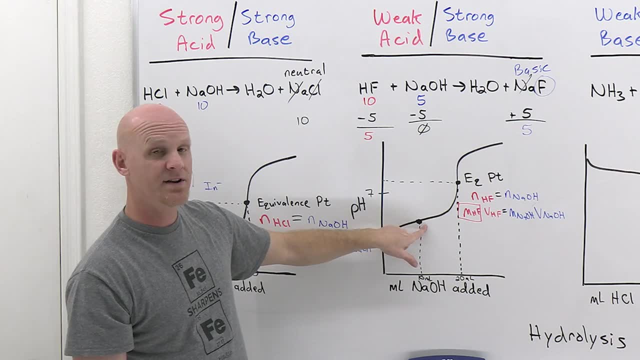 flat. the pH is right around that region. That is a buffer solution right in there. The pH is not changing a ton. So and the truth is, you got you know pKa. It turns out. this is right where the point is: pH equals pKa as well When 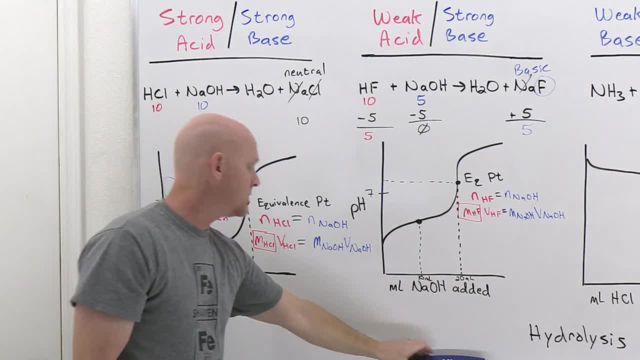 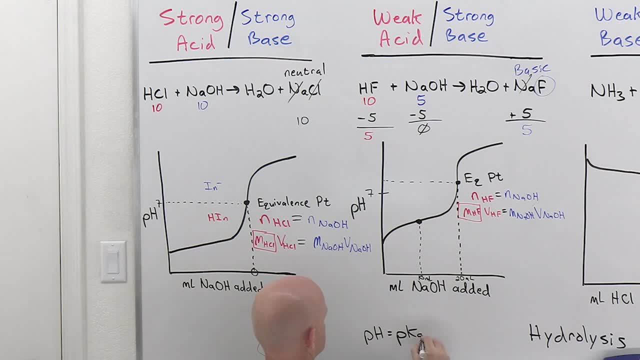 your weak acid equals your conjugate base. we learn that's when pH equals pKa. In fact, if we take a look at the Henderson-Hasselbalch one more time, real quick When your weak acid and conjugate base are equal. 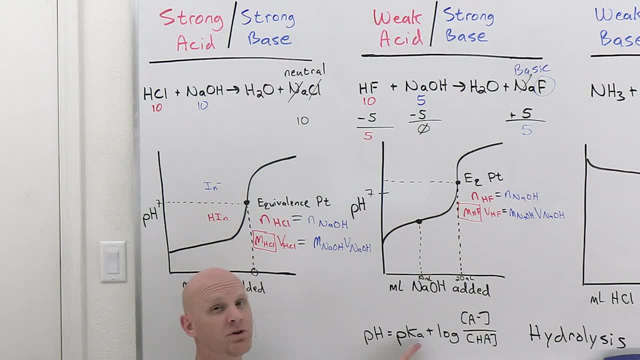 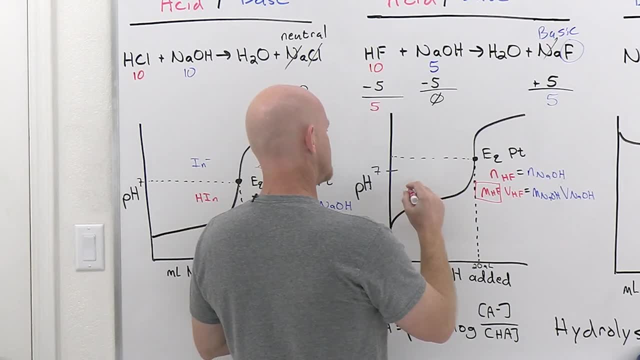 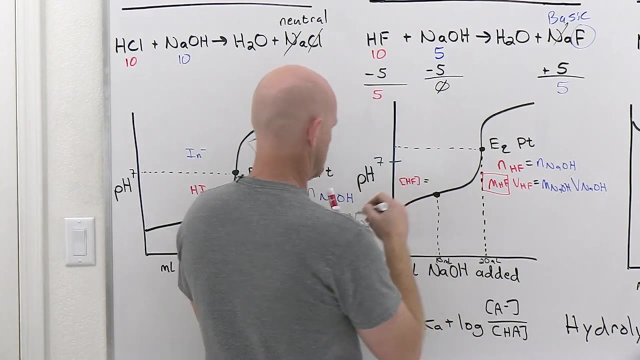 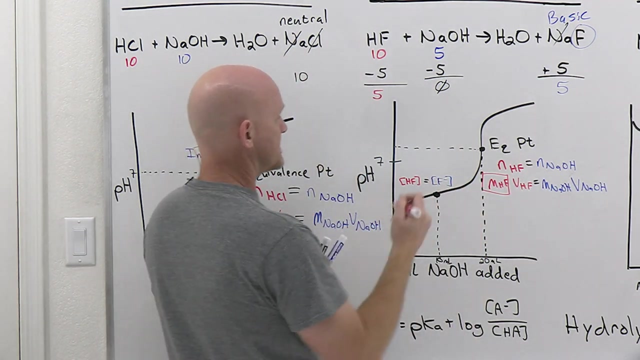 the ratio here is one, the log of one is zero and pH just equals your pKa plus zero, ie your pH is equals your pKa. And so again right at that half equivalence point, that is, where the concentration of HF is equal to your concentration of F- And as a result, that is: 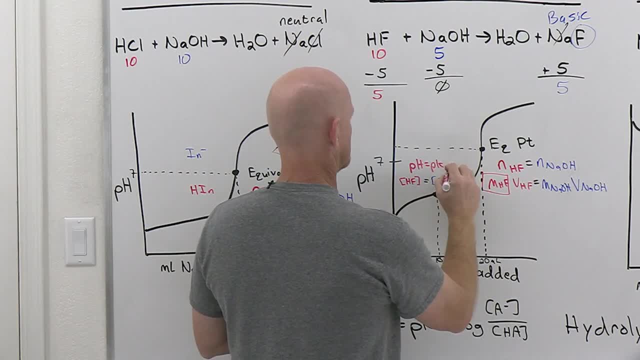 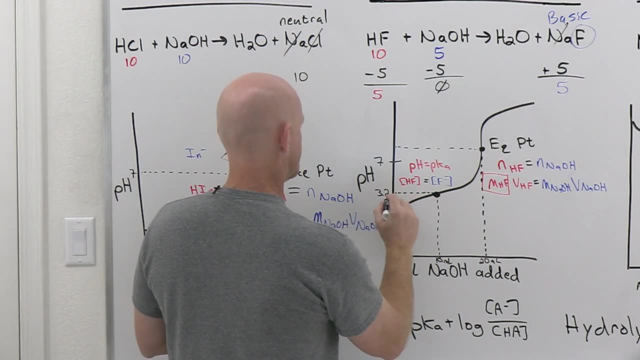 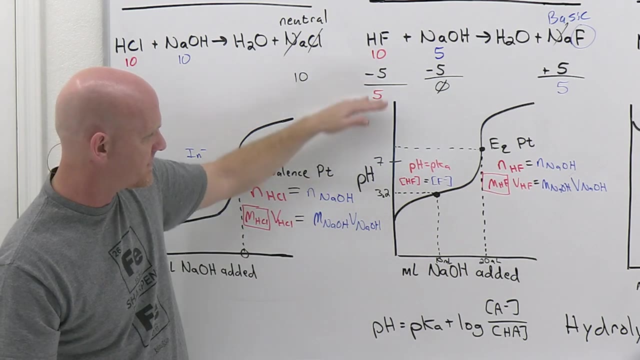 where your pH equals your pKa. pH equals your pKa. so, and we saw the pKa for HF in the last lesson and it ended up being 3.2, right around 3.2, and so if this had a, you know, nice scale on the pH scale on the left here, 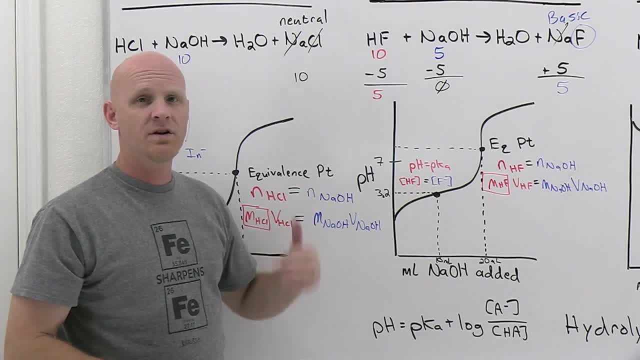 on the y-axis. then we could look at this and be like: oh yeah, pKa is right around. you know, just over 3, or maybe we'd get closer depending on how good this scale was, but it's 3.2,. 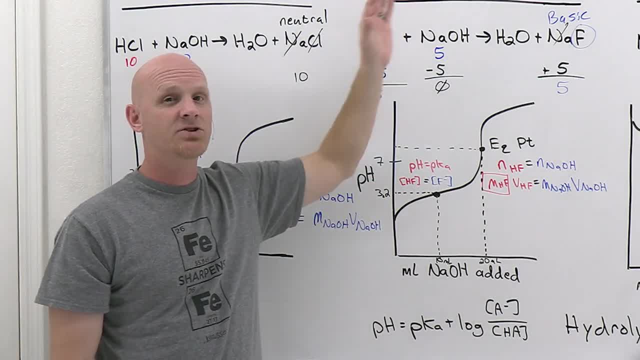 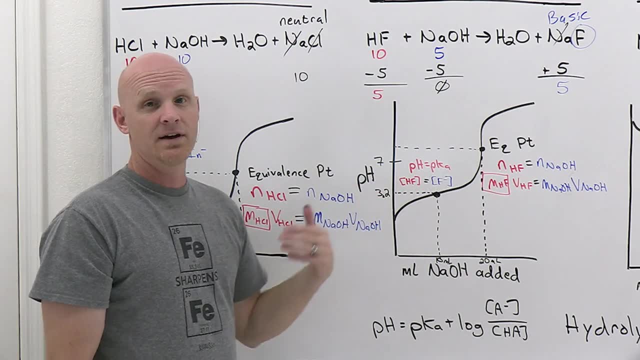 and so you can look at the titration curve of a weak acid, strong base titration, and use it not only to you know approximate what's the molarity of the HF that was in there, so but you could figure out the pKa of the acid. so in this case, you know. I said we started knowing that we're. 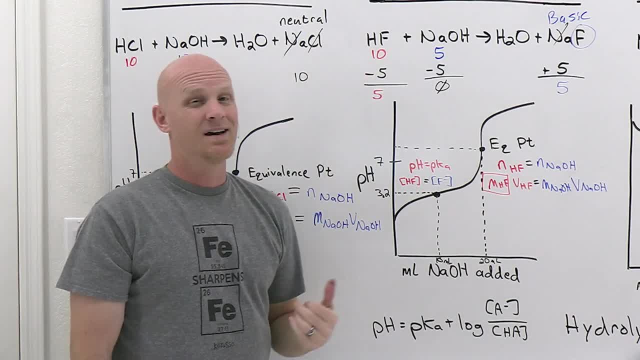 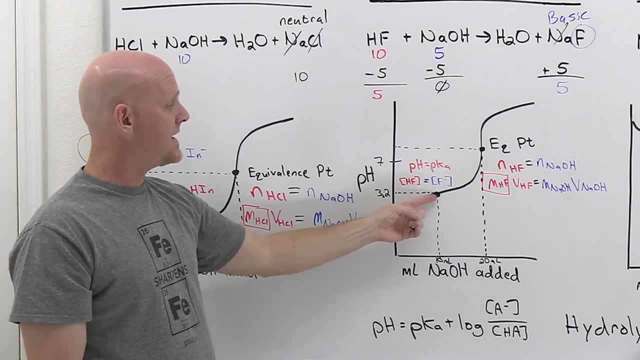 titrating HF, the analyte, with NaOH, the titrant, but oftentimes when you do a titration you don't even know what your acid is, and oftentimes you can do this and then figure out the pKa of your. 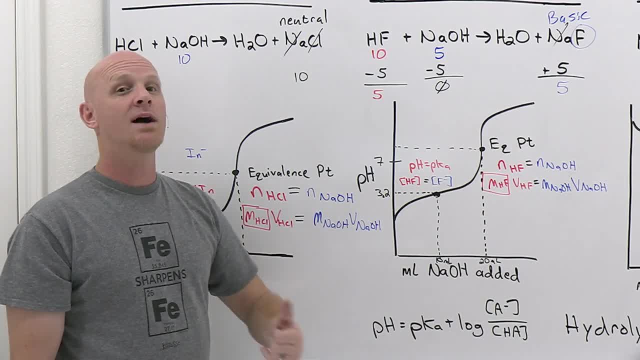 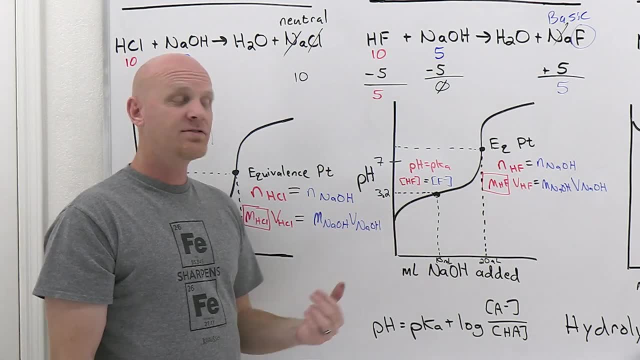 acid, and sometimes that actually can be indicative enough to help you identify what acid it might be. All right, now it turns out I said pH equals pKa and a pKa is always for an acid. so at that HF point the pH equals the pKa of the conjugate acid. 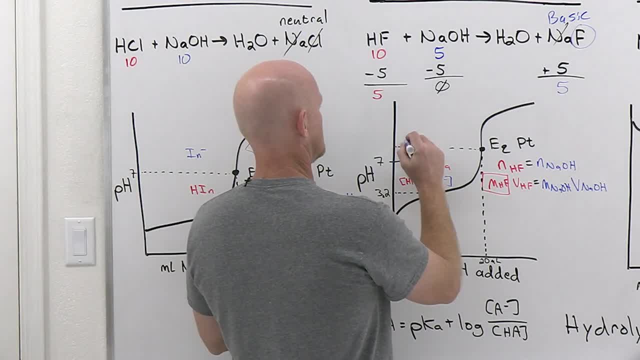 but it's also true that the pOH- let's make that look a little better- the pOH equals the pKb of the conjugate base as well. that is also true at that HF point as well. We don't usually worry. 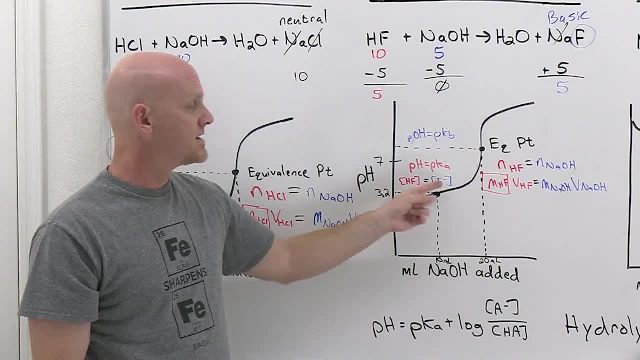 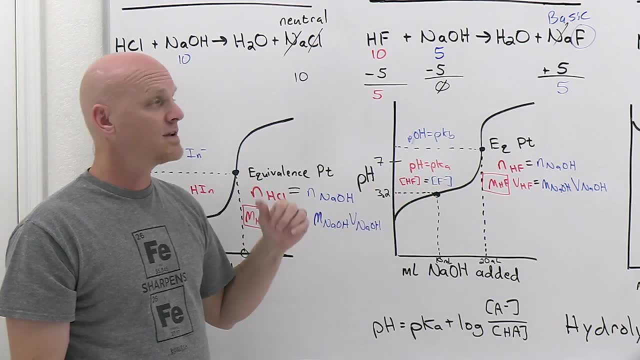 about it as much. we're usually more concerned with the pKa of the acid than the pKb of the conjugate base, but both are true. so, but in this case, in titrating a weak acid, we probably were concerned with getting the pKa of the acid, whereas in the next one, when we start titrating, 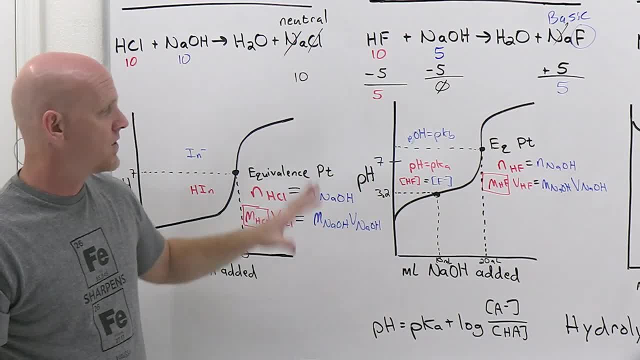 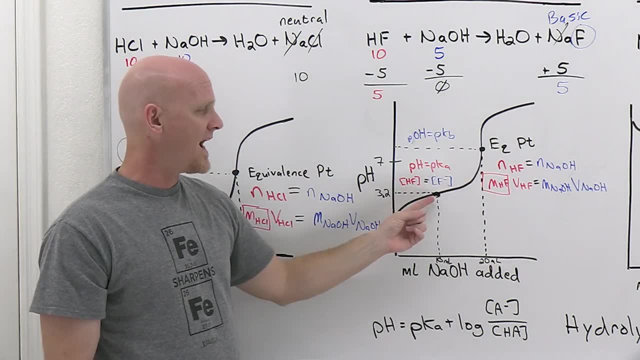 a weak base. it might be the other way around. So, but two important points on this curve, and I really want you to know the distinction between those two points. We got the equivalence point, we got the half equivalence point and a lot of students memorize them what they are. 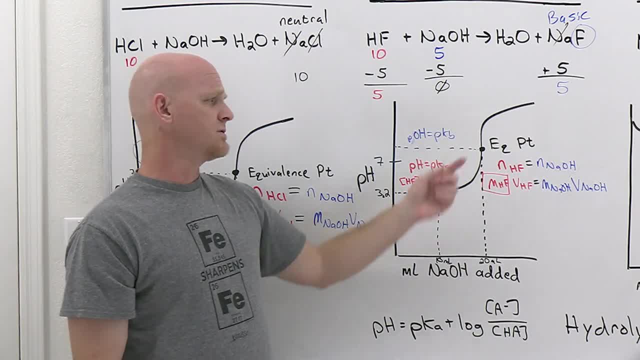 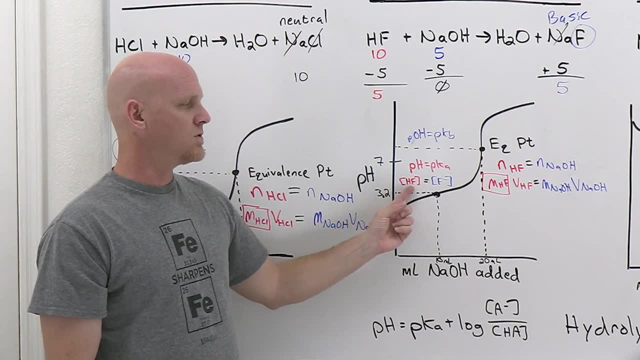 and what they mean. and they give the same definition And they say: well, at the equivalence point, the moles of acid equals the moles of base, and that's a true statement. And then they say, at the half equivalence point, the moles of acid equals the moles of base. 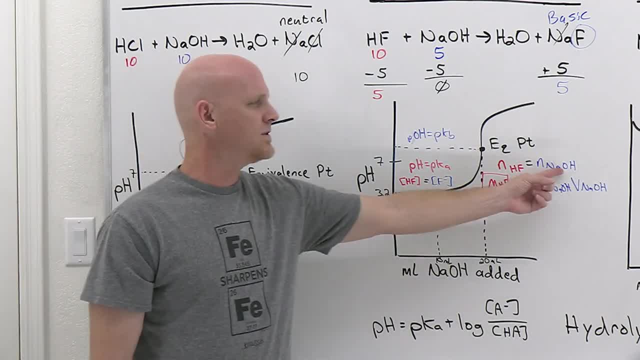 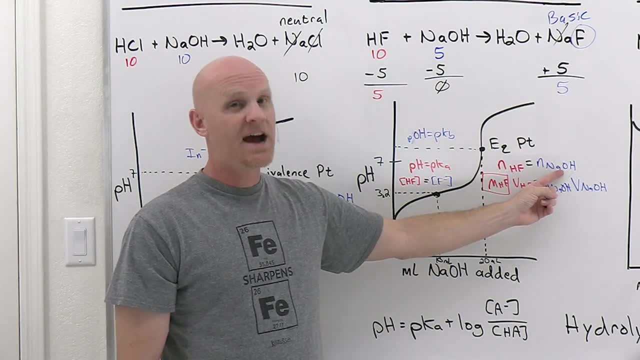 well, that's also a true statement. but we're talking about two different bases here. So at the equivalence point, the moles of the acid you're titrating, the analyte acid, equal the moles of the titrant base, NaOH in this case, whereas at the half equivalence point, 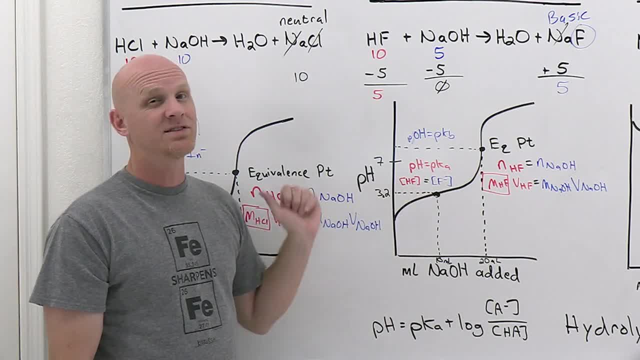 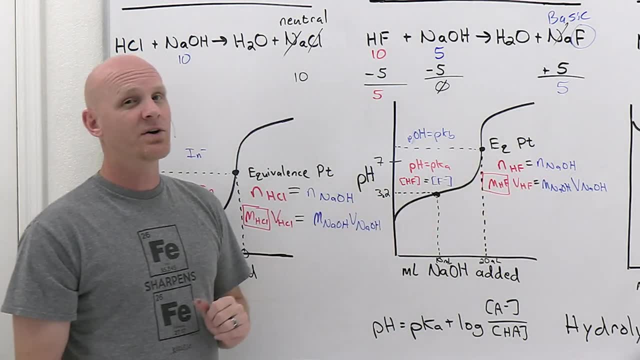 it's the moles of conjugate acid and conjugate base that are equal instead. So be careful you don't just say acid and base and not realize which base you're referring to, because it's two different bases we're saying are equal to the acid in both cases here. So hopefully, 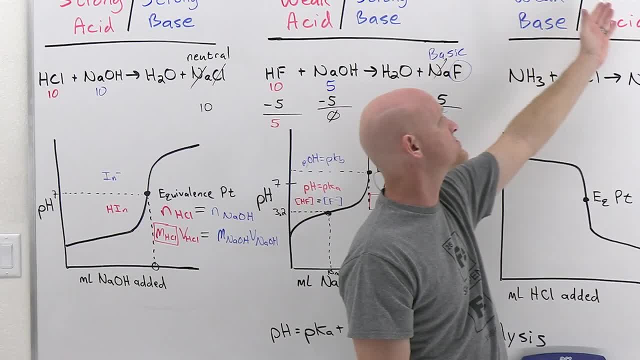 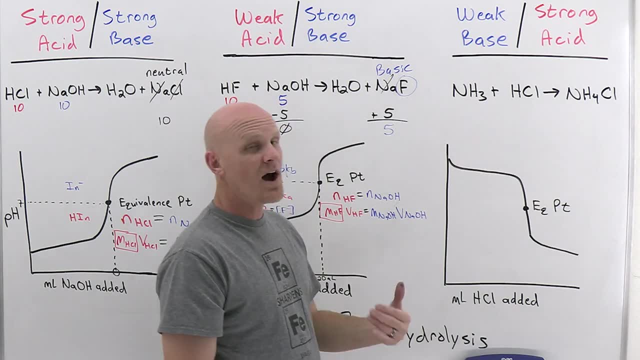 you see that distinction. Finally, let's talk about the titrate base. So let's talk about the titrate base and let's take a look at our weak base- strong acid titration. So in our weak base, strong acid titration, your equivalence point now again is not going to be seven, but it is the acid that 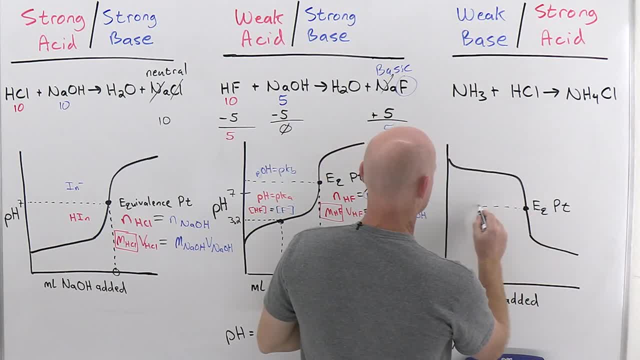 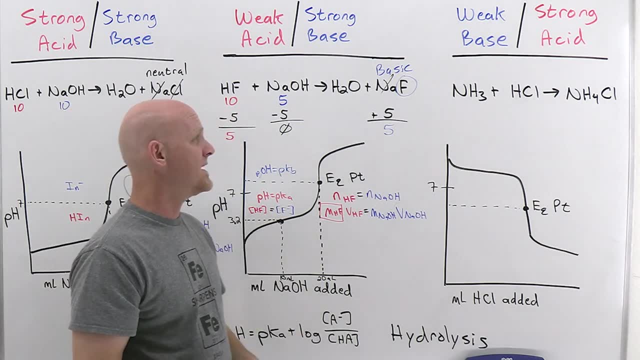 is strong, and so you're going to find out that your equivalence point is going to be a little bit acidic. It's going to be below seven now And again, usually somewhere in the four to seven range, And again the reason, though, it's not because the acid was strong, and it wins Again. 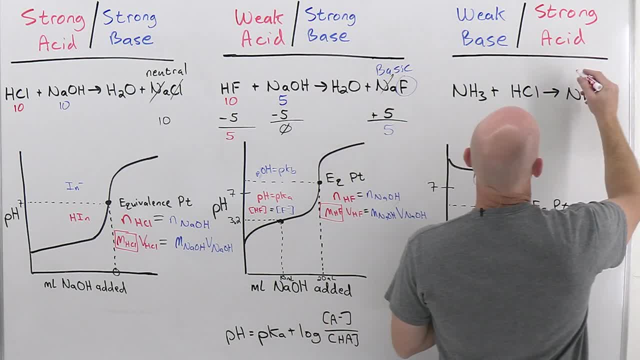 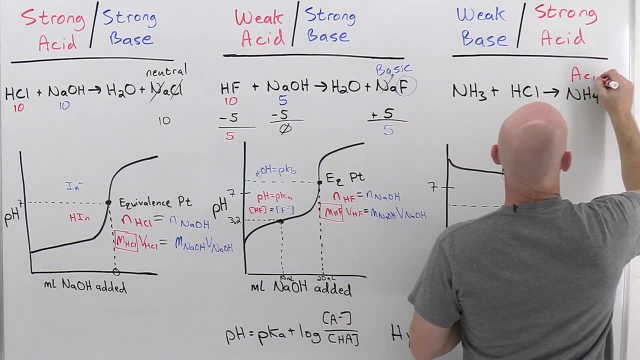 just my way of remembering it. The key is that the salt you are producing- I was going to write salt, I wanted to write acidic. Say one thing, can't write the same, All right, Can't write another anyways. So there's acidic. That's the key, The salt. 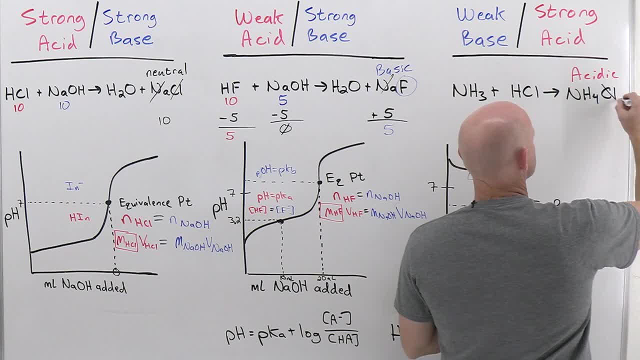 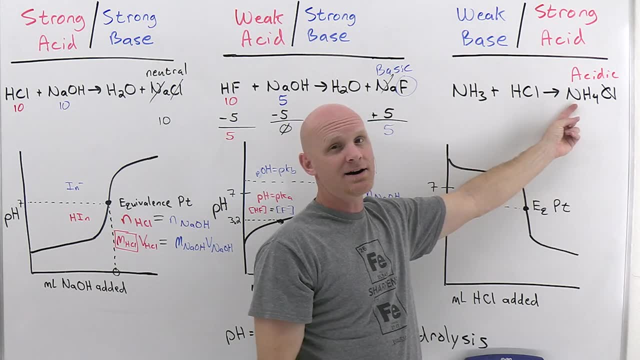 we're going to produce an acidic salt. Now again, the chloride is the conjugate base of a strong acid, so it's a negligible anion. but the ammonium is not a group one or group two metal ion or one of those rarer transition metal ions with a plus one charge. It's a polyatomic ion. It's not even. 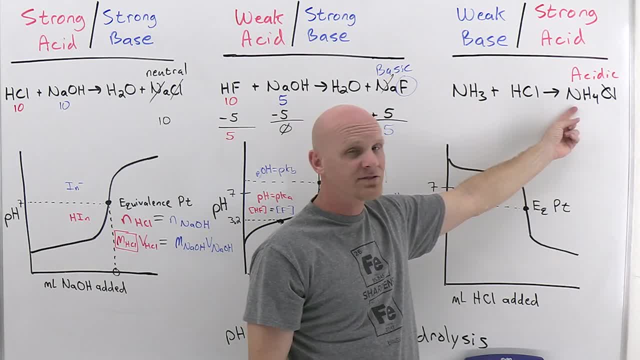 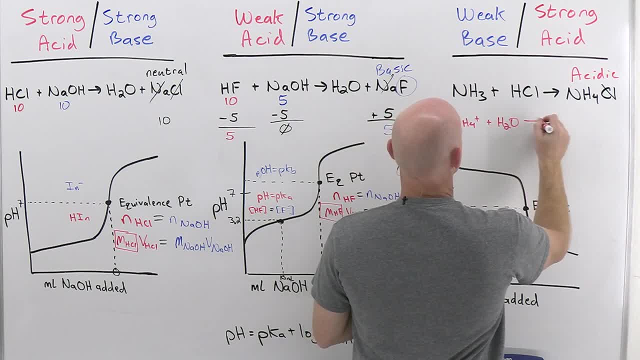 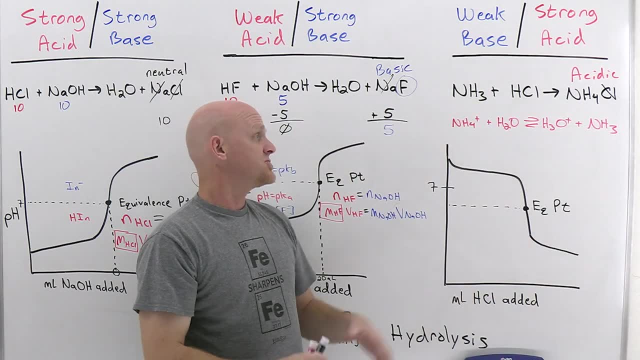 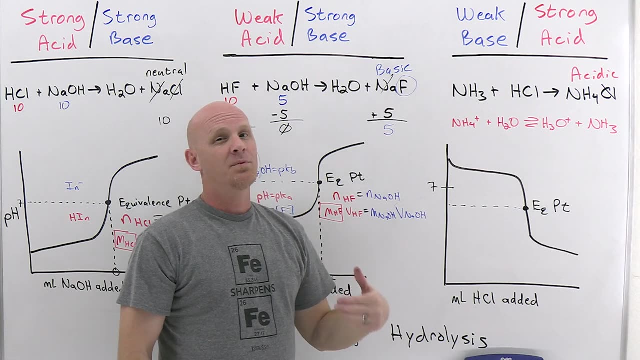 They undergo hydrolysis to produce a little bit of hydronium. And so if I asked you what is the reason that the pH is less than seven at the equivalence point in a weak base strong acid titration? A couple of correct answers. You could say that the salt. 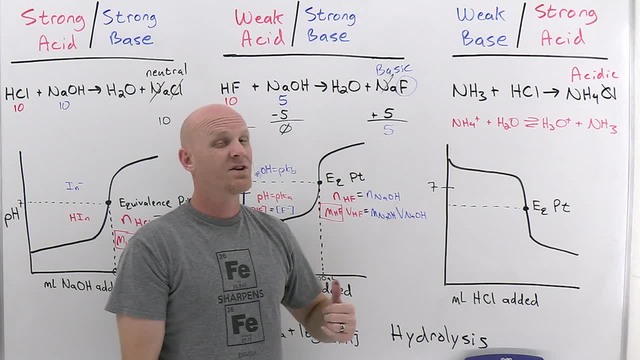 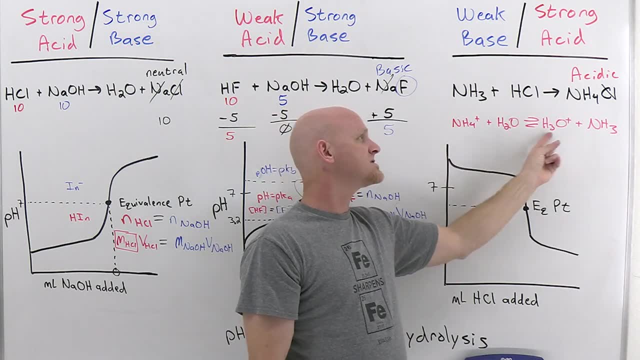 that is produced is an acidic salt. True statement. Or you could get a little more with your jargon and you could say that the salt that is produced undergoes hydrolysis to produce hydronium. That's why the pH is going to be less than seven at the equivalence point. 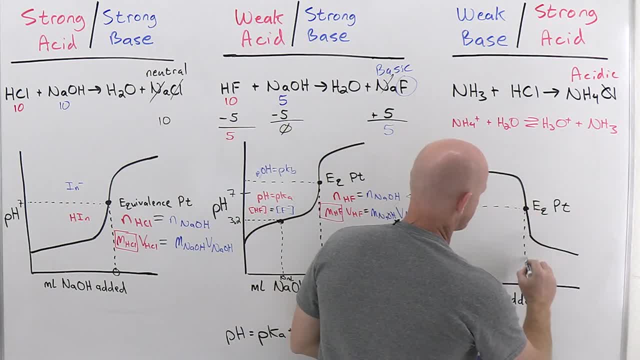 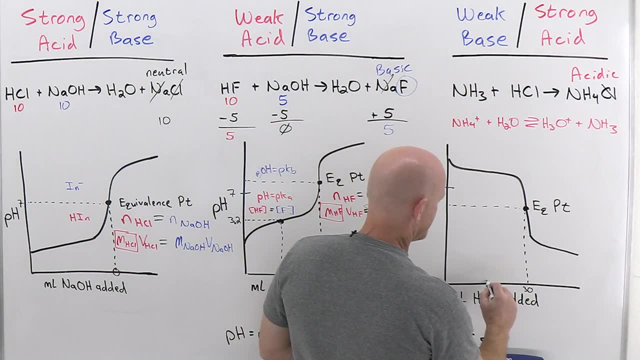 Now, once again, if you know, it took 20 milliliters or 30 milliliters or something like this, let's just pick 30, this time, 30 milliliters of our HCl, to get to that equivalence point. Well then, at the 15 milliliter mark, halfway there, 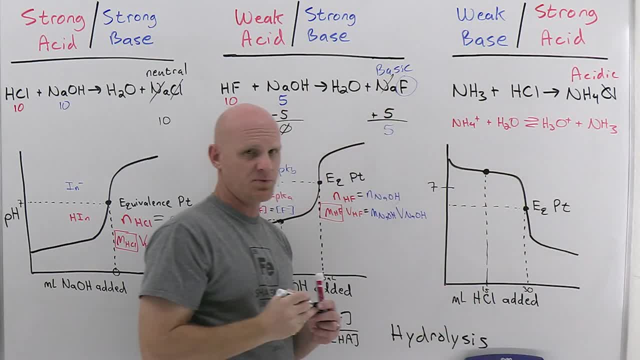 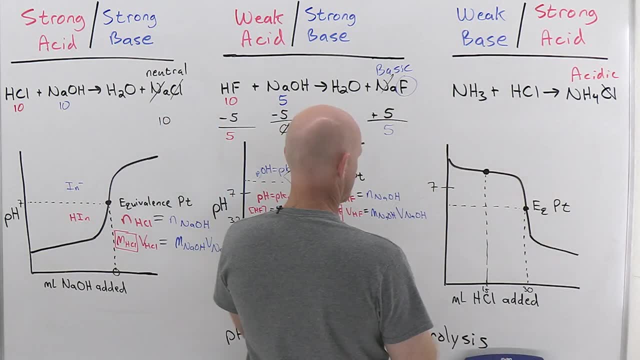 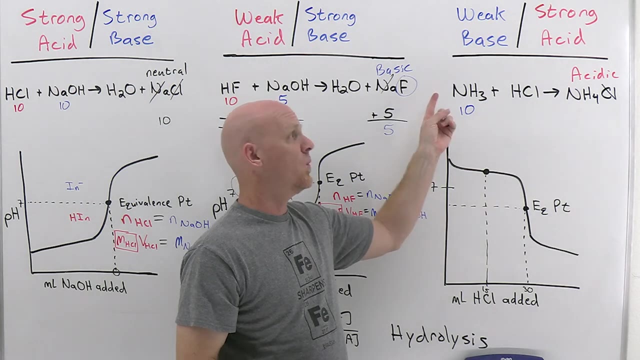 you're at the half equivalence point, And the same things were all true here that were true before. So once again, if I start off with 10 moles of my weak base, I would have to add 10 moles of HCl to get to that equivalence point. One to one ratio. So how much HCl would I have? 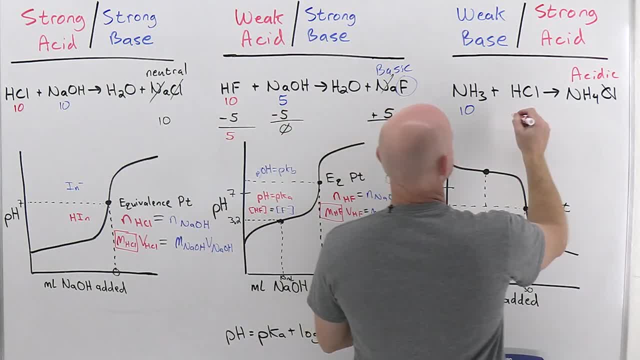 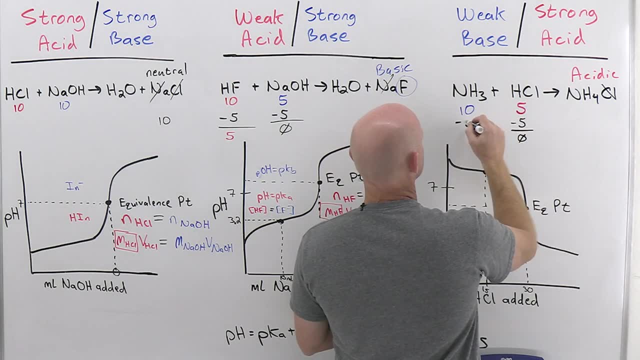 to add, to get halfway to that equivalence point, Only five moles, And that makes HCl the limiting reagent and we lose it all. And we'll lose exactly the same number of moles of NH3, but also gain the same number of moles. 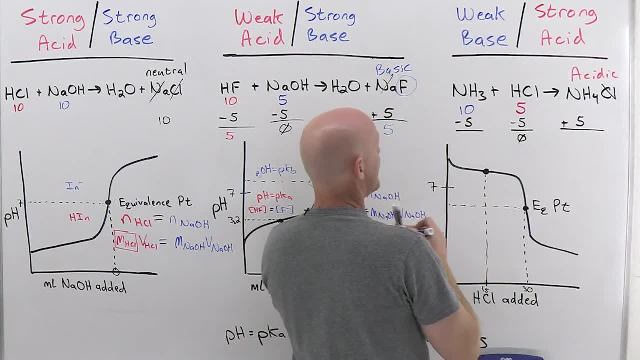 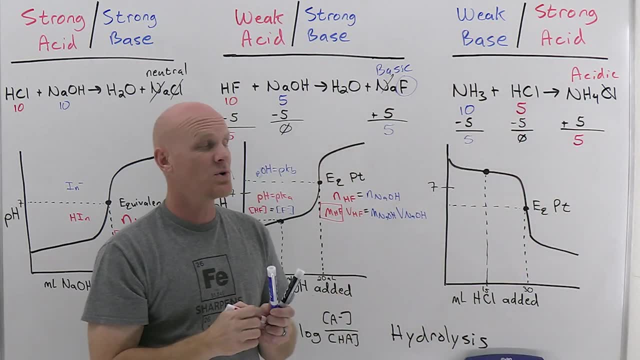 of NH4 plus the ammonium ion, And so we're still going to have five moles of ammonia left, but we'll now have formed five moles of the conjugate acid, NH4 plus, And that's why the moles of the conjugate base and the moles of the conjugate acid are going to be equal. 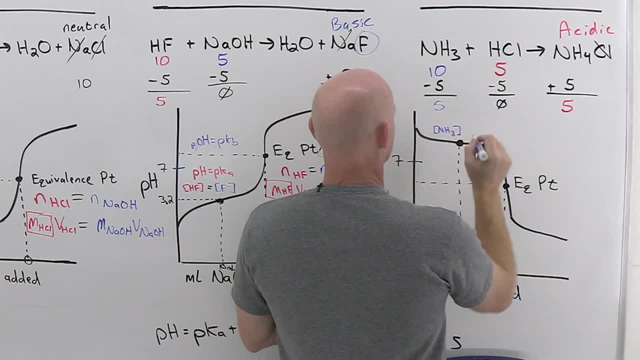 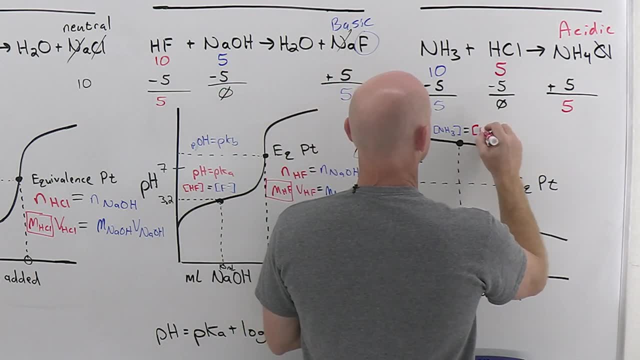 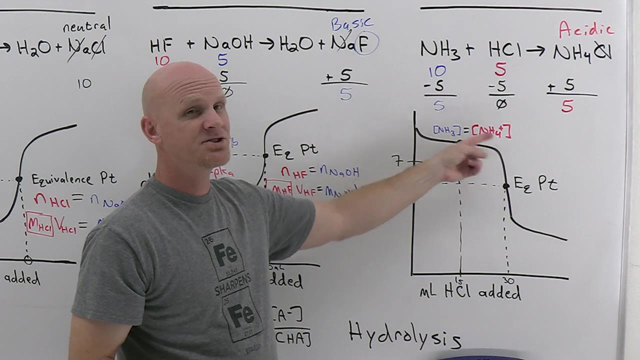 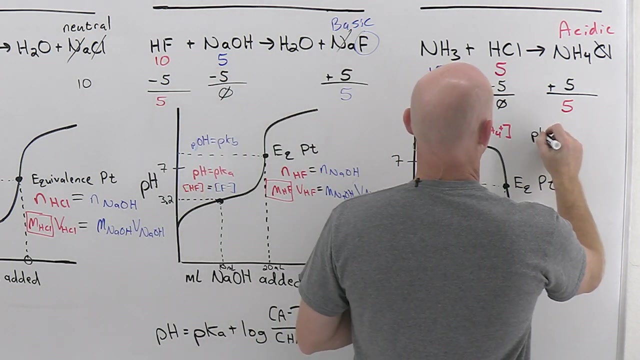 And so in this case, the molarity of NH3 is going to equal the molarity of the ammonium ion as well. So, and as a result, once again, if your conjugate acid and conjugate base concentrations are equal, well, again that happens when pH equals pKa, And again, always true as well is that pOH. 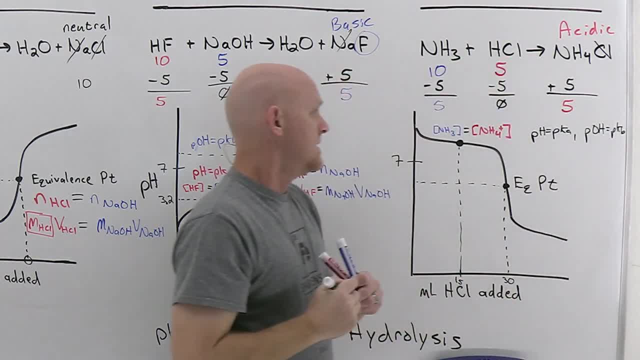 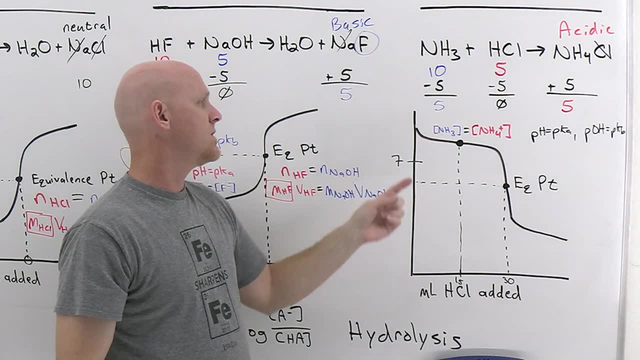 equals pKb. So if your goal was to get the pKa of ammonium, great, you're good to go. If your goal was to get the pKb of ammonia, well then, rather than looking at the pH, you'd want to convert it. 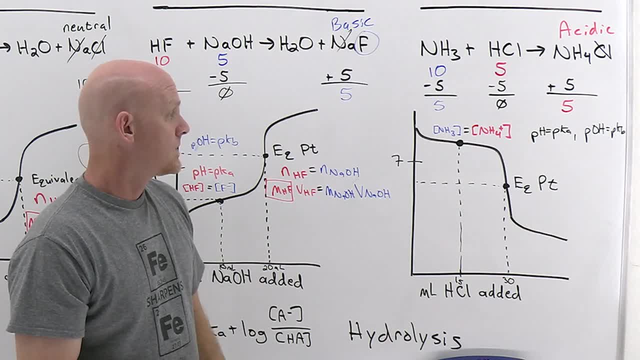 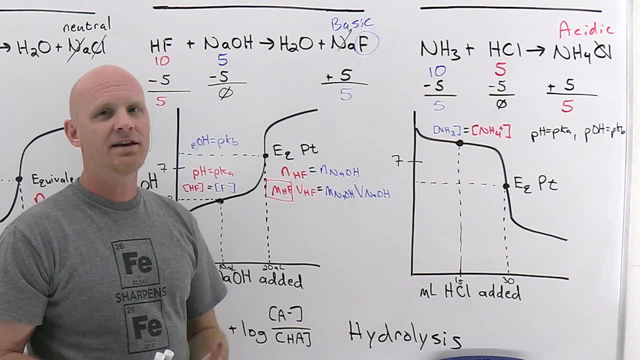 into a pOH instead, Cool. So one thing to note on this one. this is: you're much less likely to see a base getting titrated. It's just usually kind of, you know, secondary to talking about acids getting titrated first. So, and when students do see it, though, they're like so is the half. 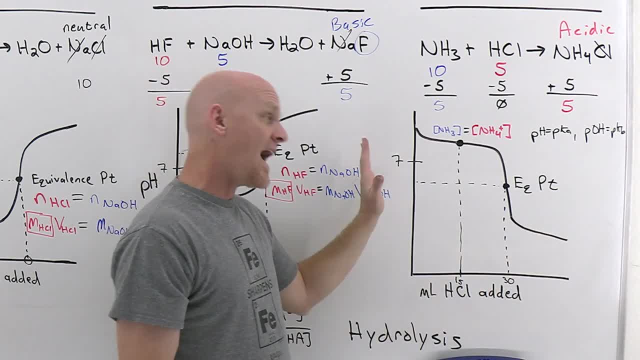 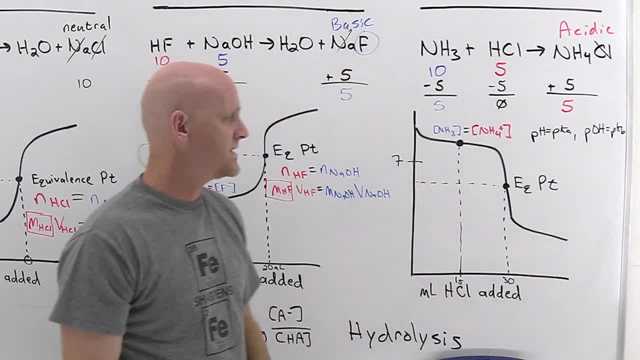 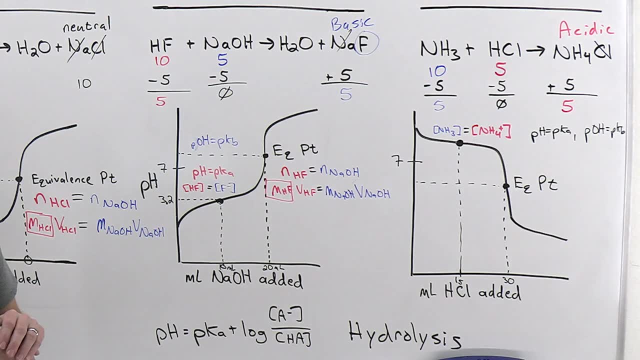 So you definitely don't want to have a pKb of ammonia. So you definitely don't want to have a pKb of ammonia past that equivalence point. It's definitely before Cool Once again, since your weak acid and conjugate base concentrations are equal right there. 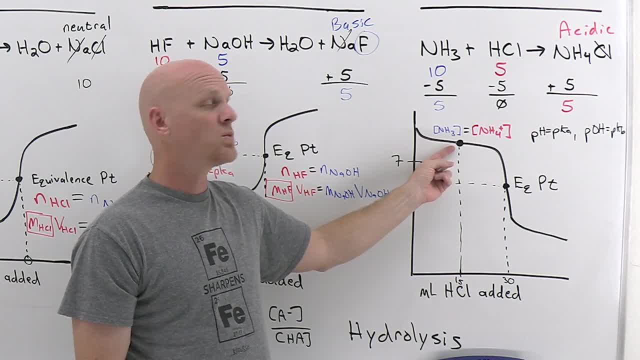 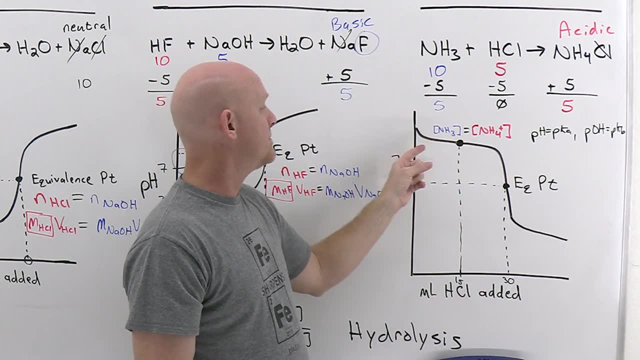 that again is right, where pH equals pKa and you have a buffer once again. And again you can go one pH unit higher or one pH unit lower and the pH doesn't change a whole lot. but get outside that region and the pH jumps. Get right outside that region and the pH will jump in one way shape. 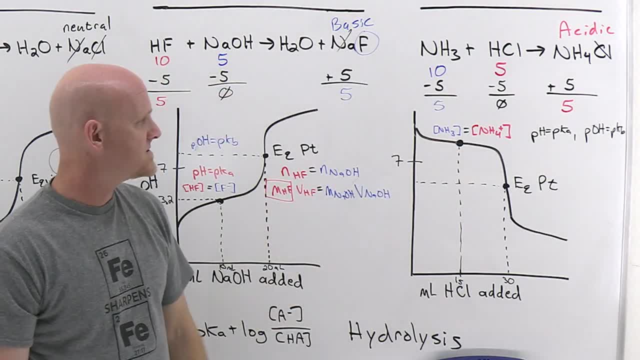 or form and it's no longer going to have a pKa of ammonia. So it's going to change. So you don't have to have a pKa of ammonia, You don't have to have a pKa of ammonia longer, a buffer. And so once again on this titration curve, there's a couple of interesting